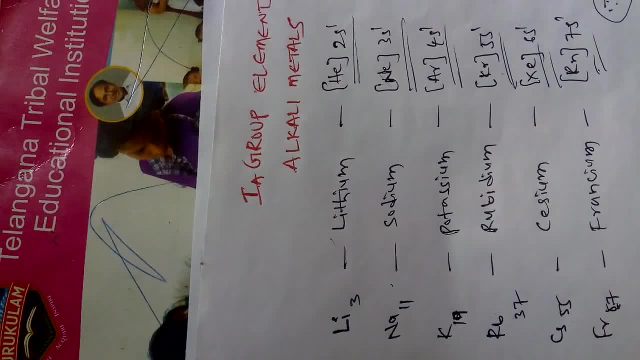 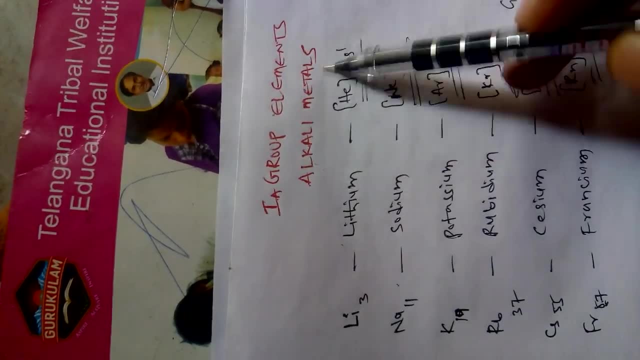 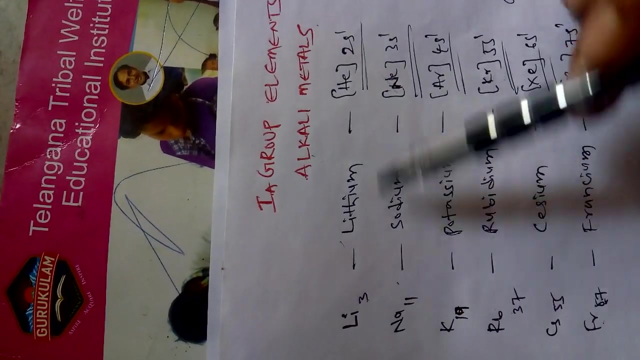 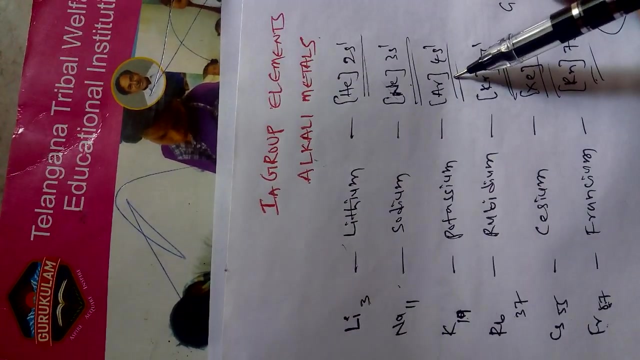 So now we are discussing about first A group elements In this first A group group elements. first A group elements are known as: like alkali metals, The lithium, sodium, potassium, rubidium, cesium potassium are belongs to first A group elements. This lithium electron configuration is helium 2s1, sodium electron configuration is neon 3s1, potassium electron configuration is argon 4s1 and rubidium electron configuration is krypton 5s1 and cesium electron configuration is helium 2s1. 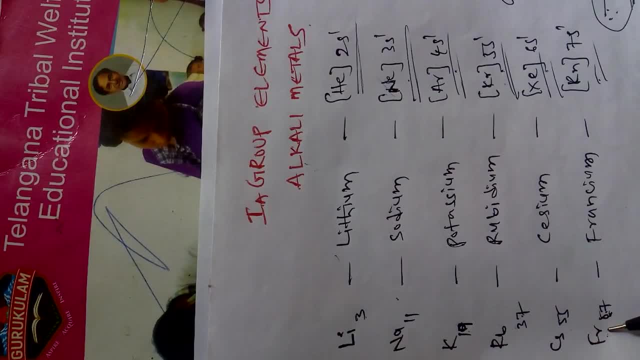 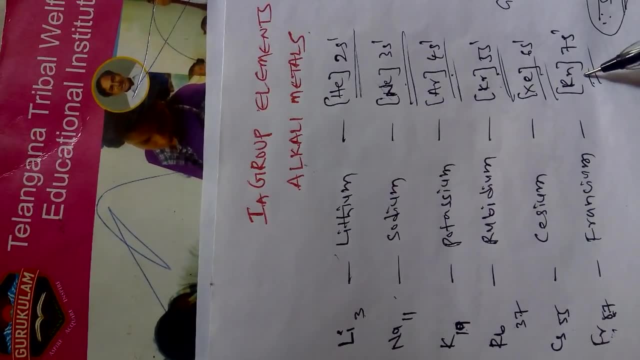 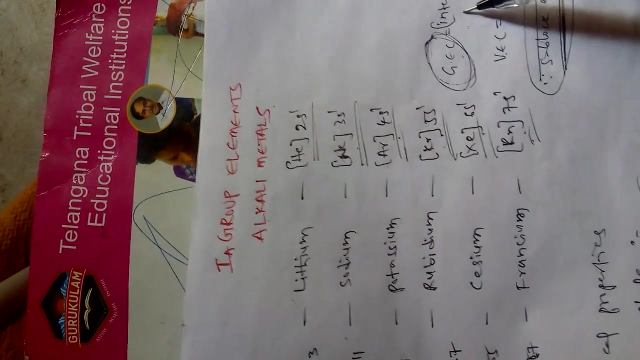 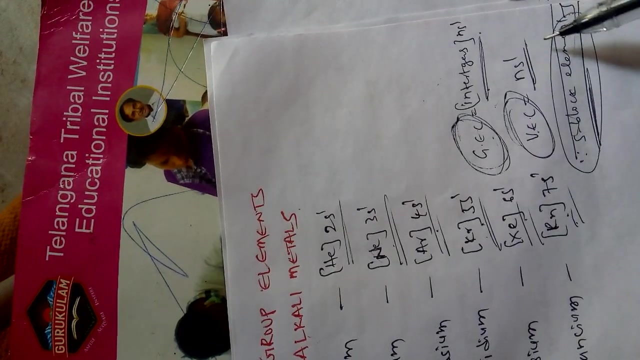 Second electronic configuration is xenon 6s1. and last, finally, radioactive element, that is francium. electronic configuration is radon 7s1.. Okay, here what happening? this general electronic configuration, This general electronic configuration is like inert gas and ns1.. This valency electronic configuration is like ns1.. Okay, it means inert gas. ns1 is a general electronic configuration. 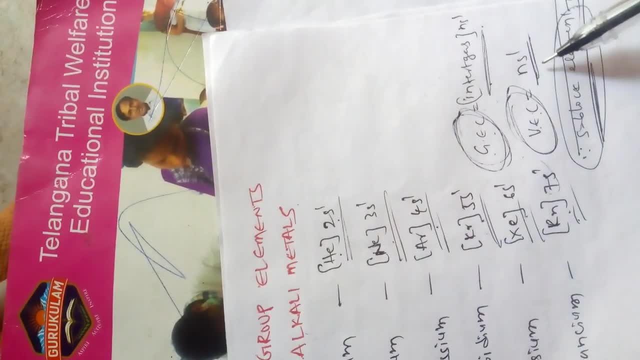 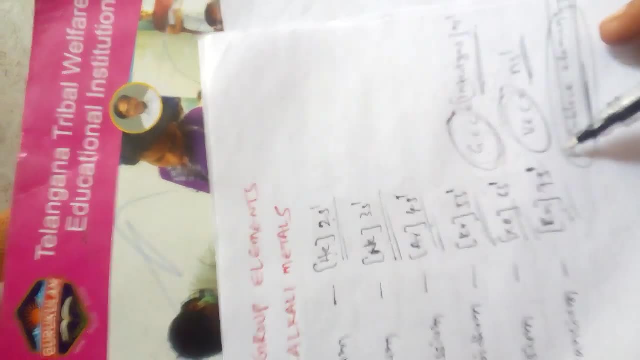 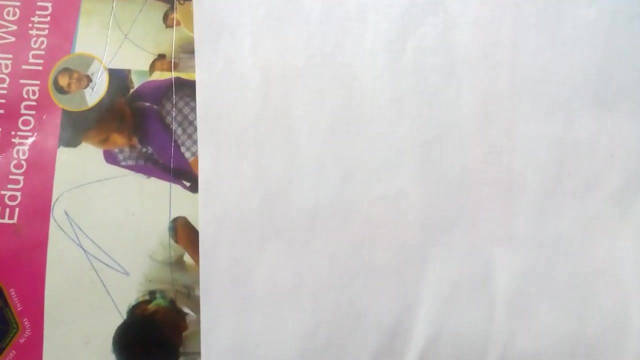 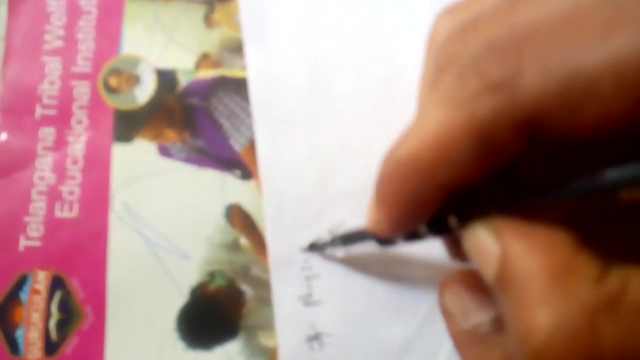 These ns1.. Okay, it is a valence electron configuration, So here the differentiating electron enters into only s block, So these are belongs to, of course s block elements. Okay, so when we are discussing about any topic, just we need to know some fundamentals regarding that. here. for first, A group elements. here fundamentals are like physical properties and chemical properties. 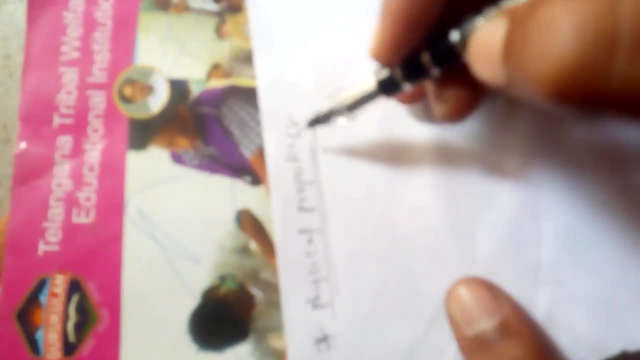 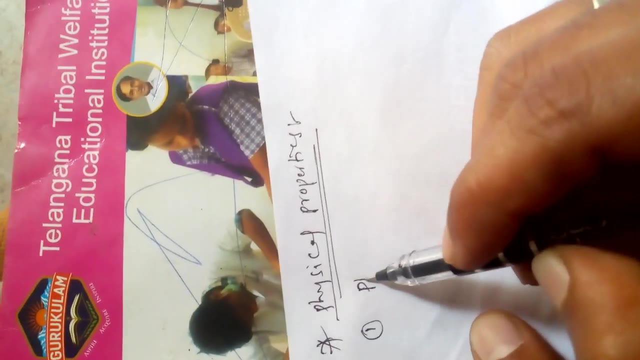 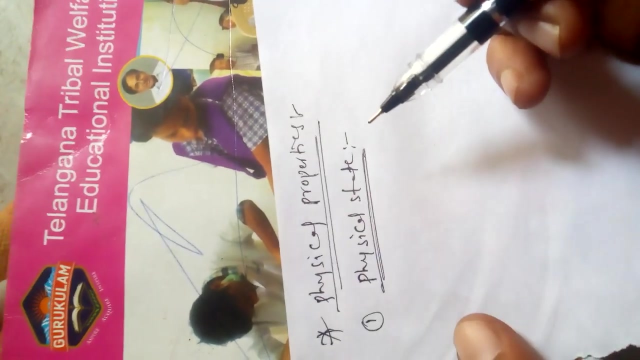 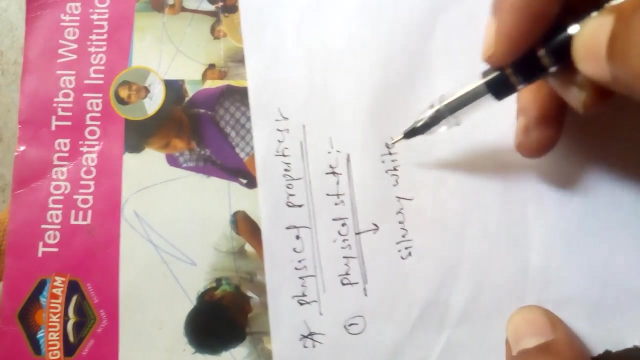 Now we are discussing about physical properties. don't bother about handwriting, please. Here physical properties now, first of all, and discussing about physical state Appearance. okay, physical state means like appearance. these are looking like silvery whites- Silvery white. As well as these first a group elements are soft metals. 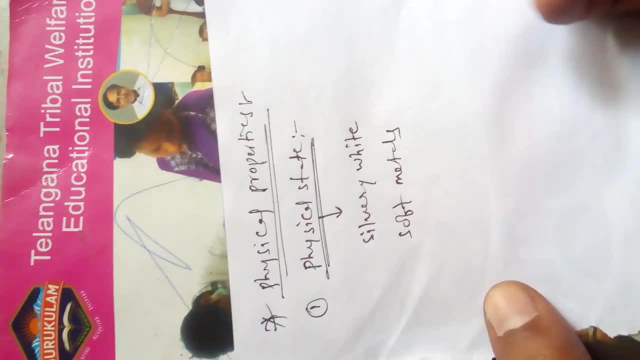 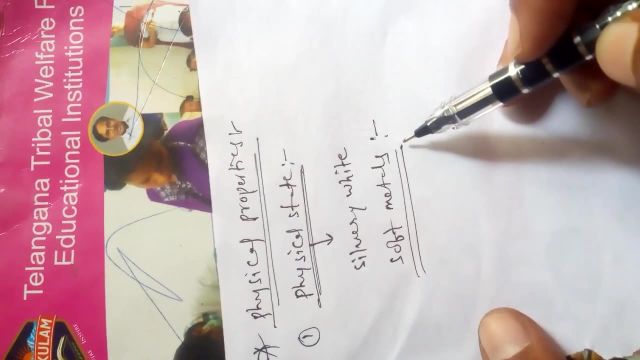 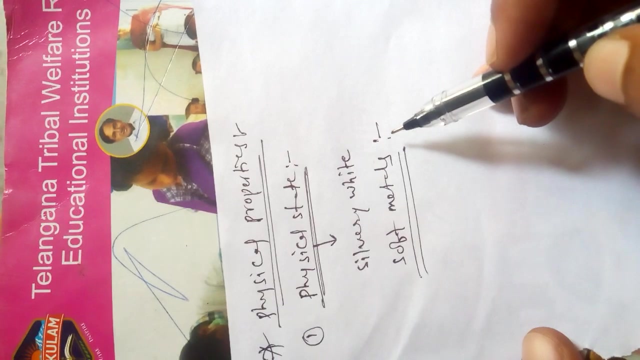 Okay. so here are. Okay, these lithium, sodium, potassium, rubidium, cesium, francium, are soft metals, and it means soft metals like these metals can cut with the help of knife or blade like that. Okay, so this softness is due to presence of weak metallic bond. 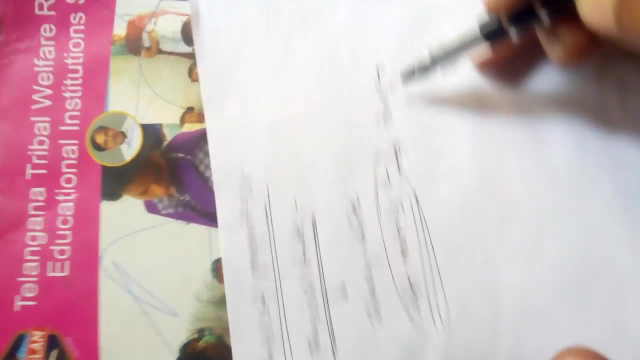 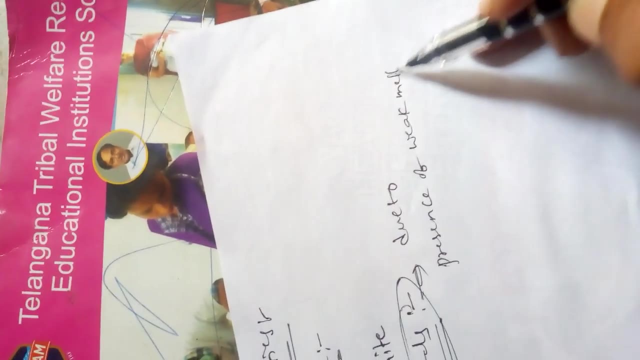 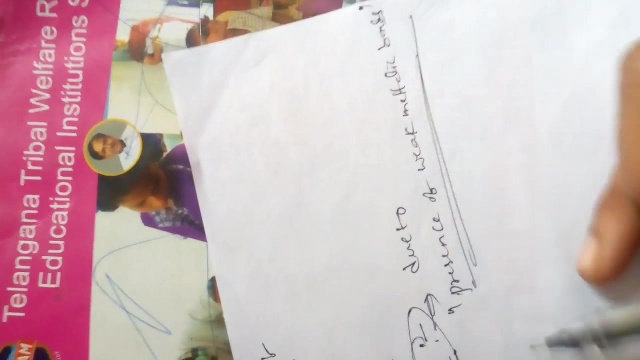 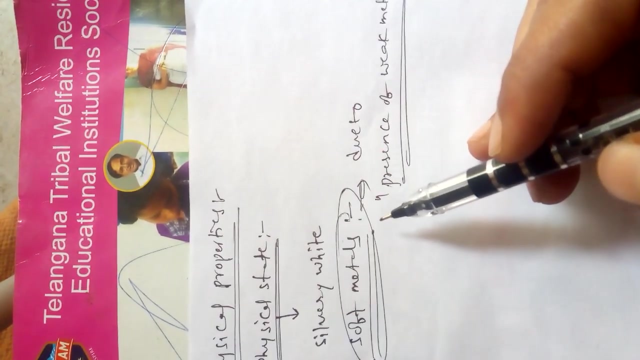 These softness is due to presence of weak metallic bonds. Due to presence of weak metallic bonds, this softness is increases and how it is: silvery. white means like due to mobile valence electrons. due to mobile valence electrons, it is looking like this: 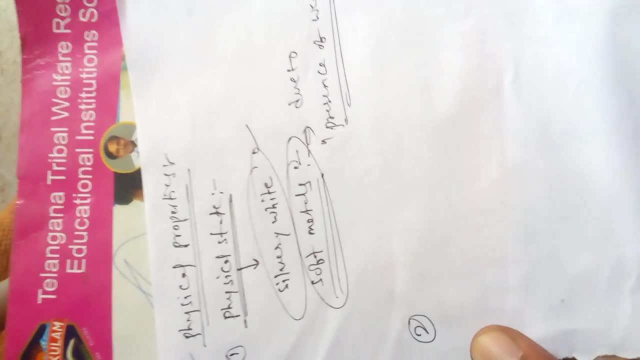 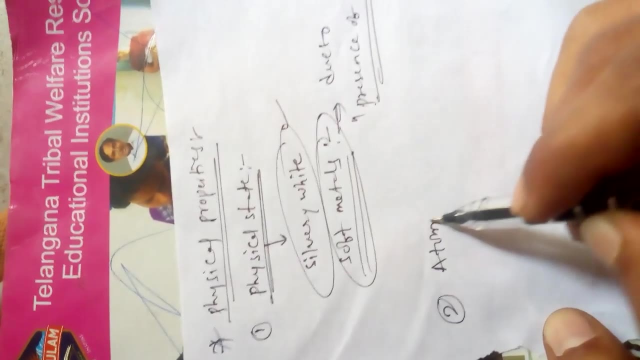 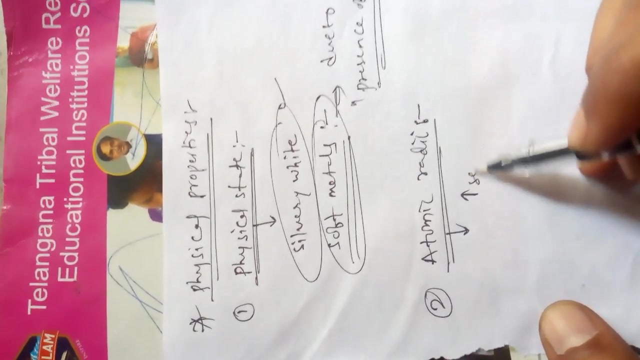 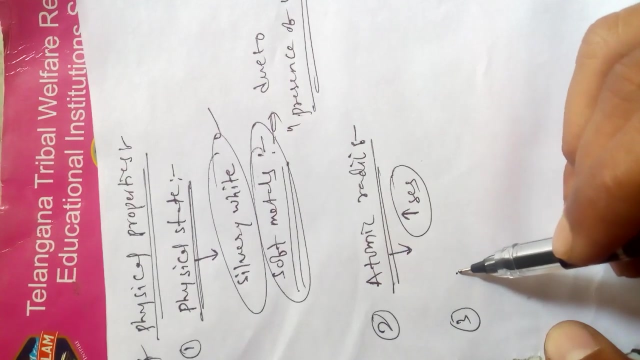 These are the physical state and appearance. and second property is like atomic radii: Moving down the group, what happens? Atomic radii increases, Okay. third property is like atomic radii. After atomic radii it is ionic radii. 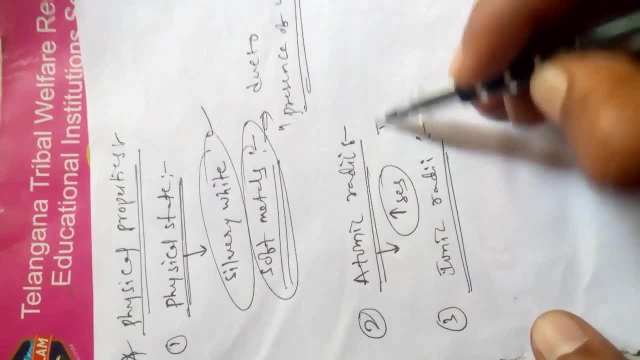 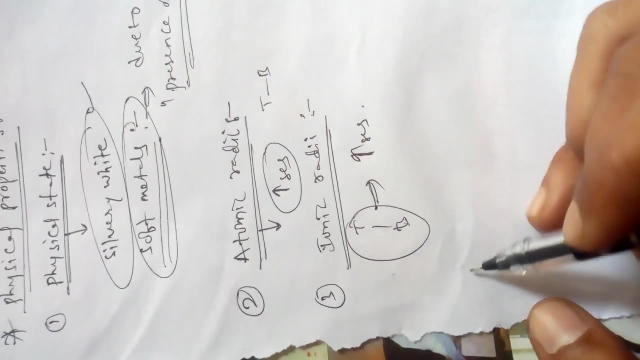 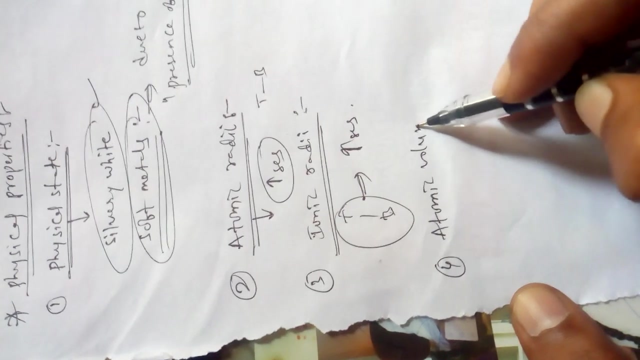 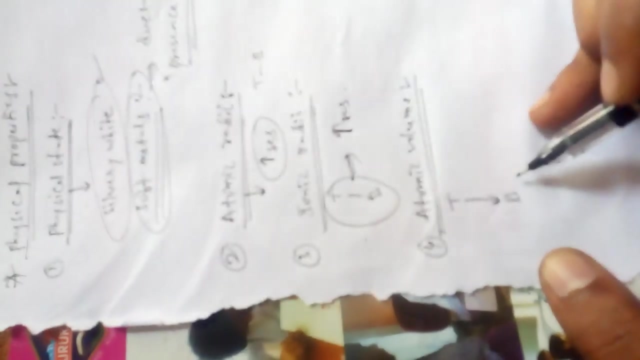 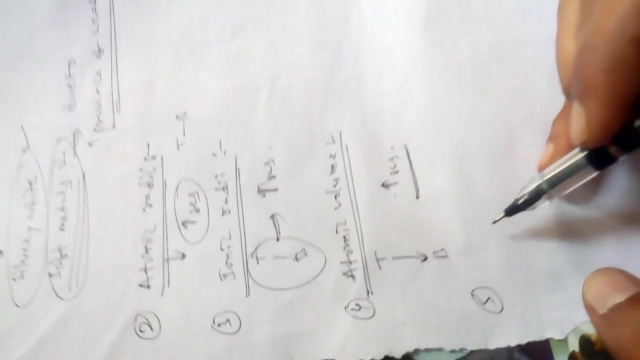 Definitely, if atomic radii increases, it is like atomic radii, It increases. when top to bottom- Here top to bottom also- ionic radii definitely increases. Then fourth property is atomic volume. Atomic volume, What about atomic volume When the top to bottom? top to bottom means lithium, sodium, potassium, rubidium, cesium. From the top to bottom, atomic volume also definitely increases, Okay. and fifth property is like: 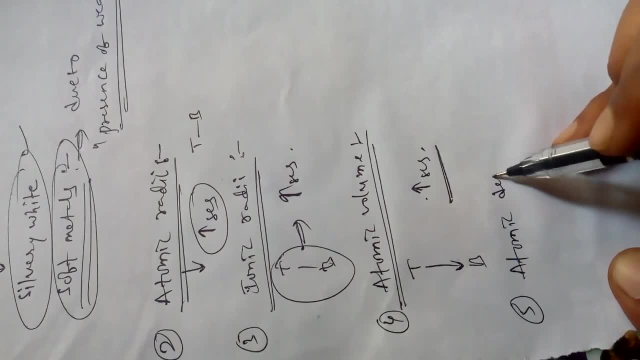 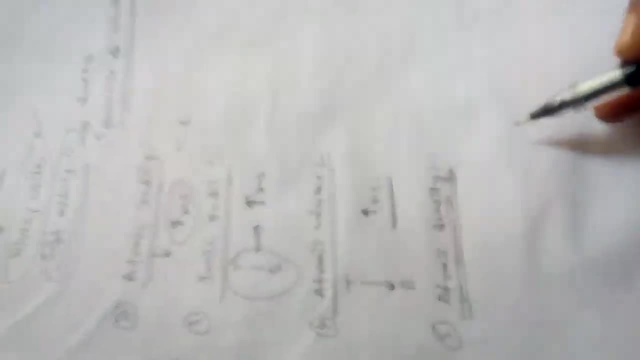 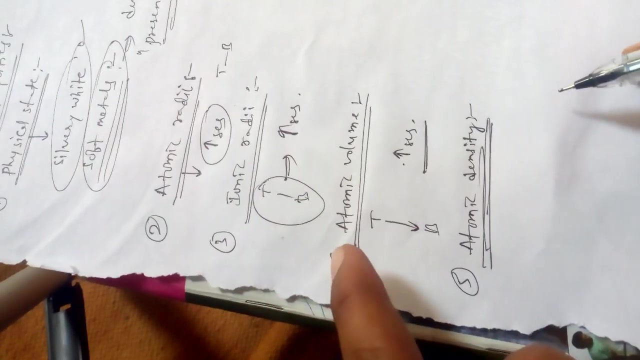 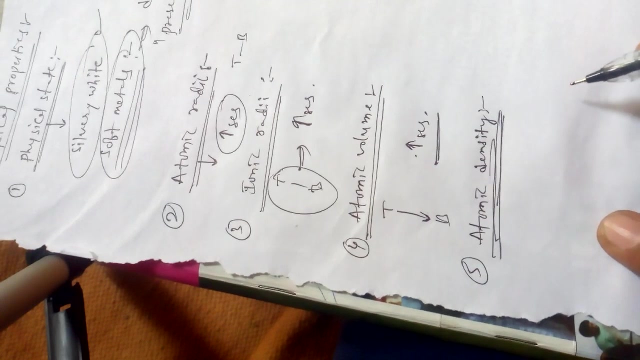 atomic density, Atomic density- Here Some exceptions also are there Here in atomic density. Please listen carefully. Actually, what happens When ionic radii and atomic radii atomic volume is increases? definitely we assumes like top to bottom it should be increases with respect to increasing weight. okay. 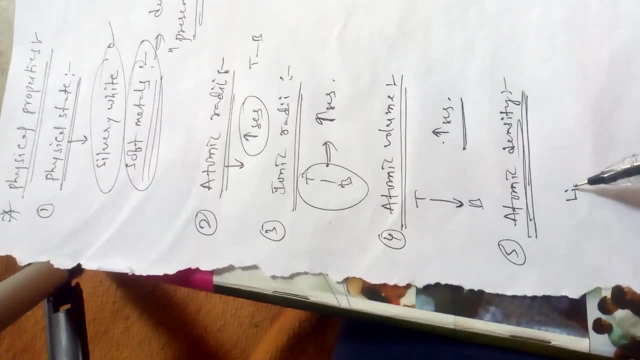 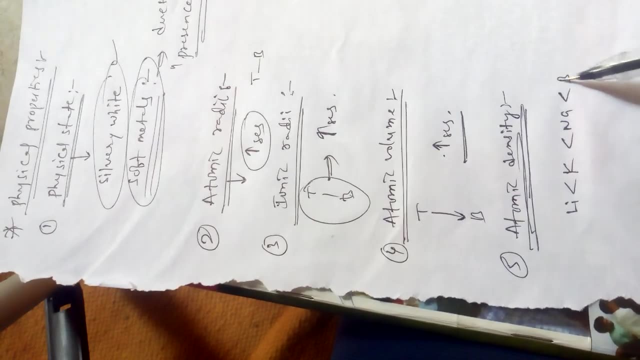 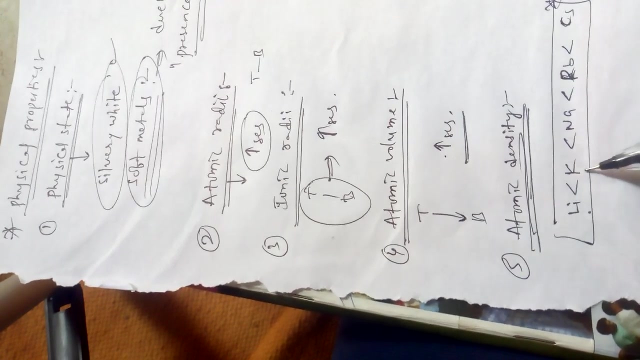 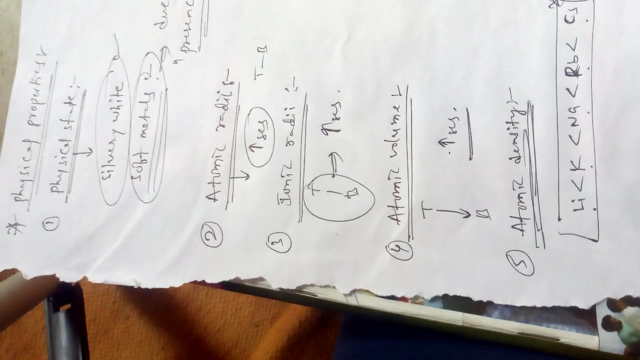 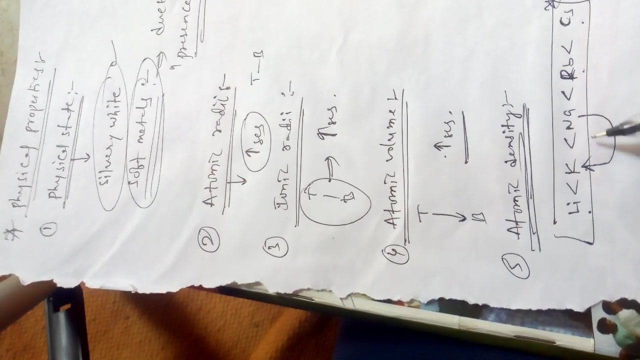 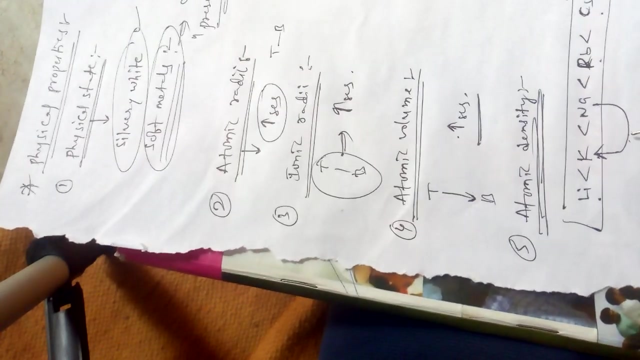 So, but here, What happening here? The order will be like lithium, potassium, sodium, rubidium and cesium. What happening here? Lithium, potassium, sodium, rubidium, cesium- Okay Here, top to bottom increasing. but here, exception is: sodium is less, greater than potassium. Potassium is less than sodium. Okay Here, potassium is less than sodium. Okay, Potassium is less than sodium. This is the exception case. 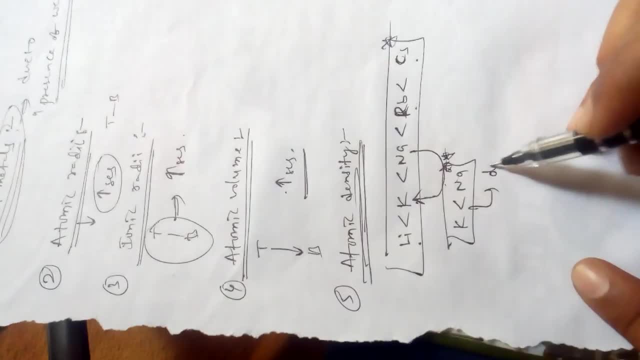 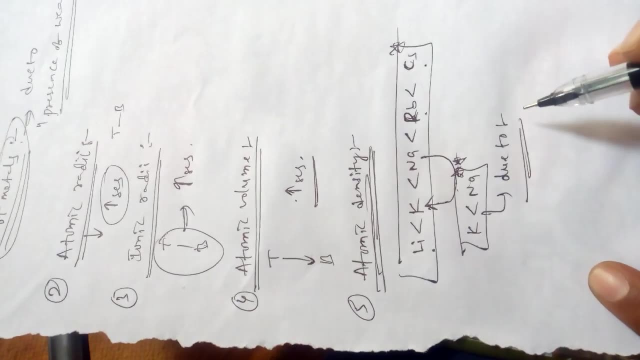 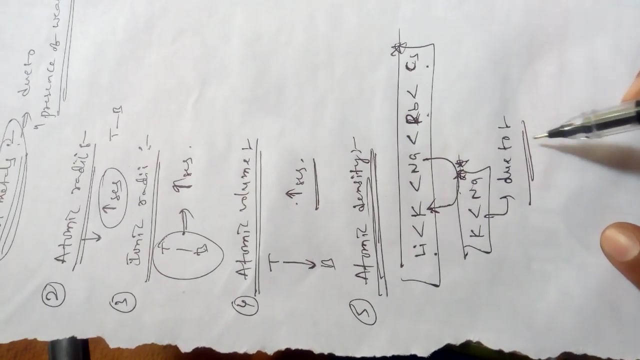 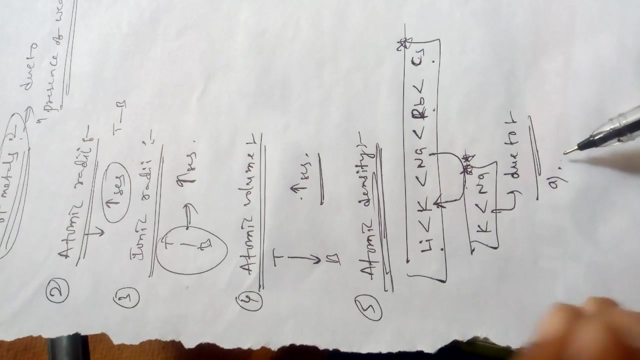 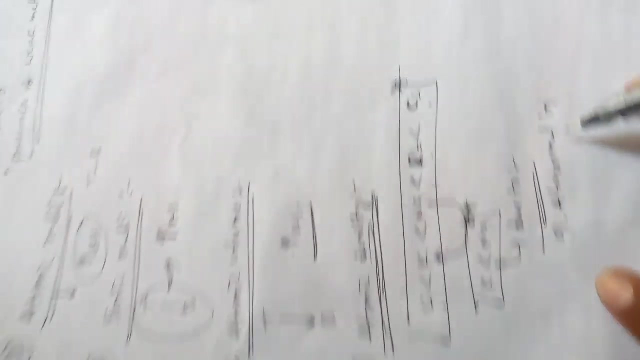 And it is only, it is only due to like why potassium? potassium is less than sodium means only because of abnormal increase in size. potassium is increases size abnormally, so that's why, and as well as potassium having it present a violence inner energy shell, also so due to abnormal increase in size. abnormal increase in size and as well as. 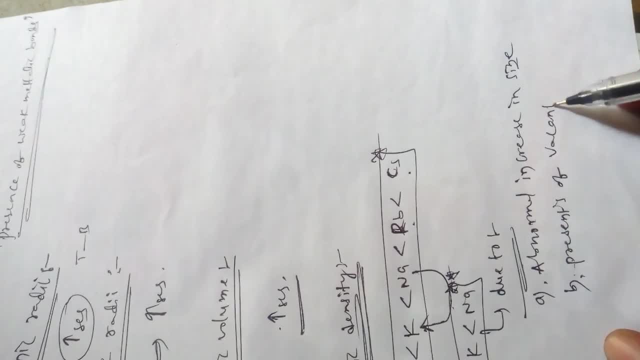 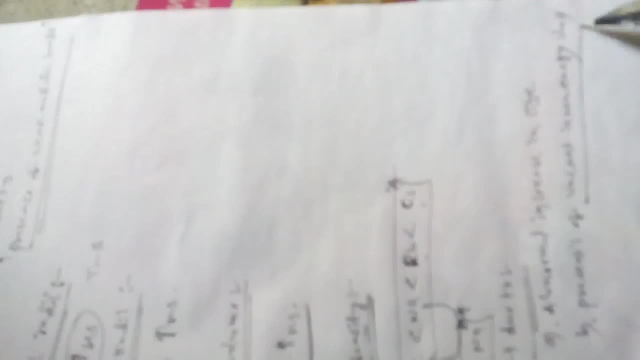 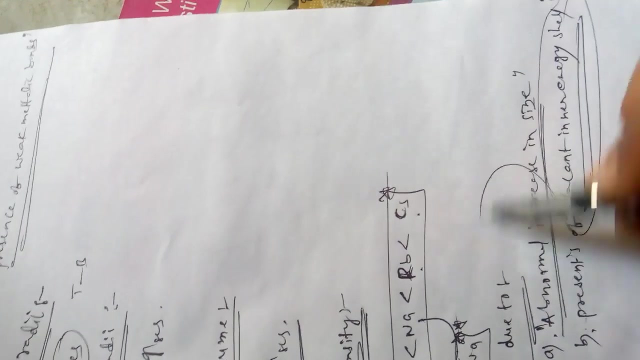 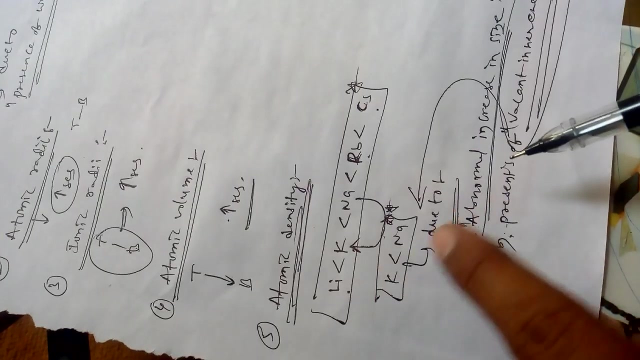 presence of vacant inner energy shell, presence of vacant energy energy shell in potassium and abnormal increase in size. the potassium is less than sodium. okay, here exception is in atomic density. in atomic density, actually, uh, top to bottom increases. it should increases, but here the exception case is potassium is. 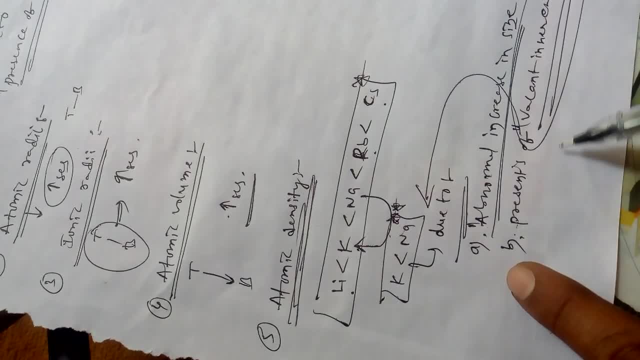 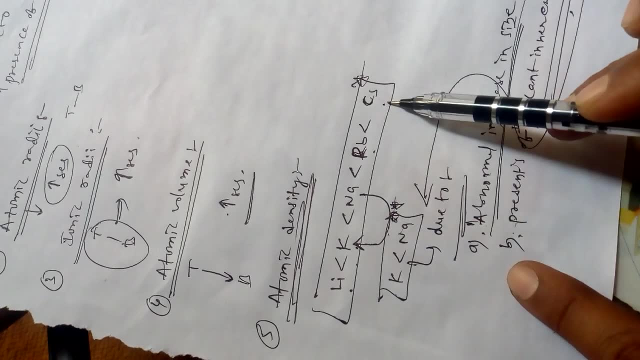 having less than sodium. it is due to abnormal increase in size and as well as presence of vacate inner energy shell in potassium. so, due to this, atomic density order will be like this: okay and um. this is the fifth property and sixth property is uh- ionization energy. 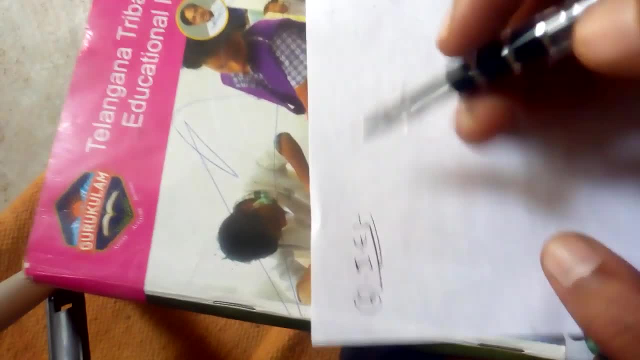 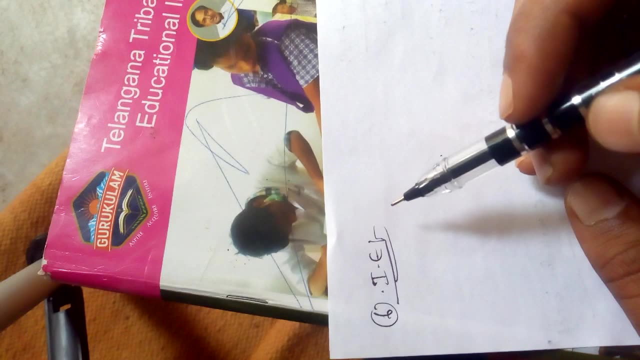 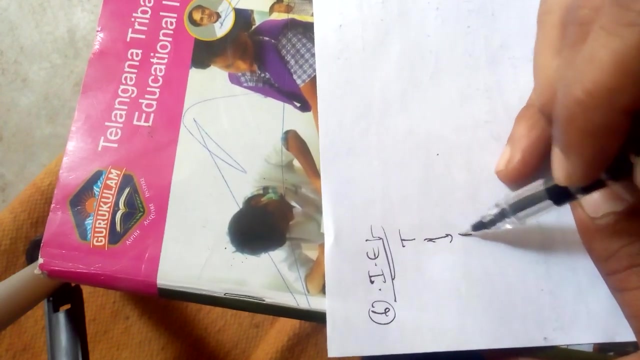 ionization energy- ie, i'm writing like a shortcut- ionization energy. of course, ionization energy means, like uh, removing of electrons, required energy for removing of electrons, so required energy for removing electrons. uh, moving down the group. it means top to bottom. what happens top to bottom? definitely, definitely increases. uh, decreases. 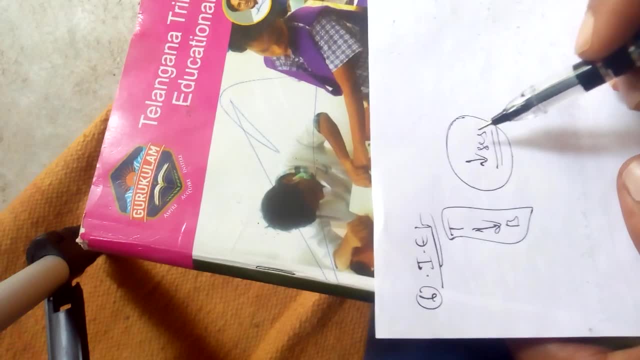 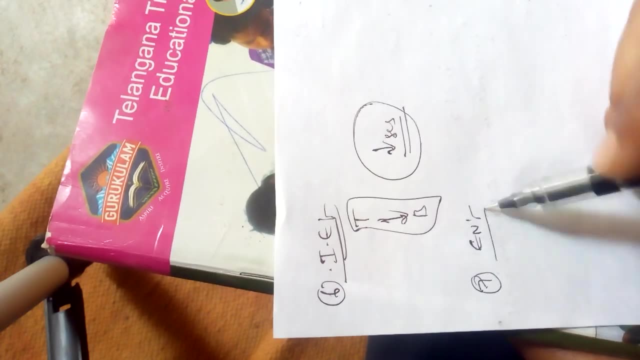 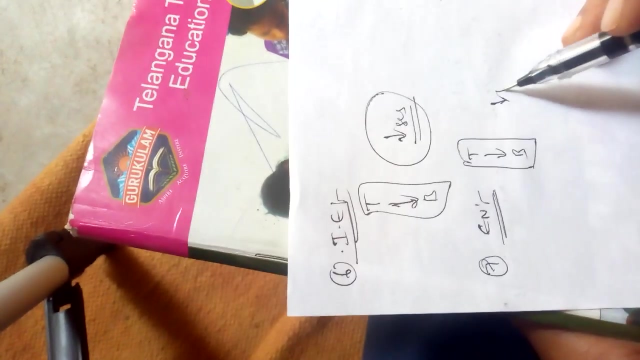 okay, top to bottom definitely decreases. and seventh property is like uh electronegativity. we know that uh, top to bottom electronegativity. um, electronegativity top to bottom decreases and as well as left to right increases. okay, and here, opposite of electronegativity, that is. 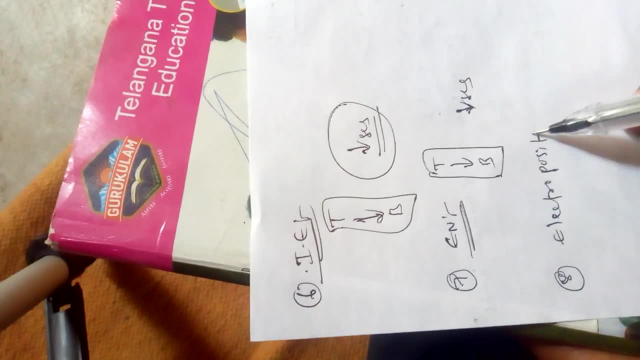 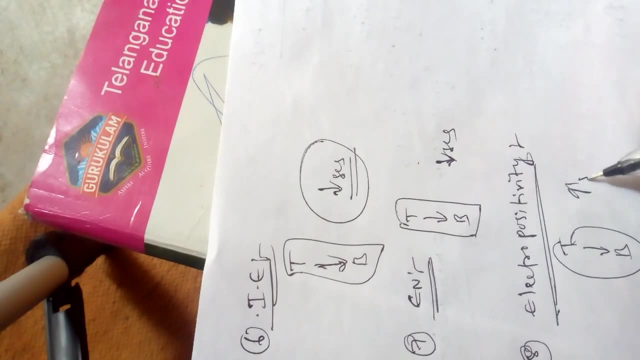 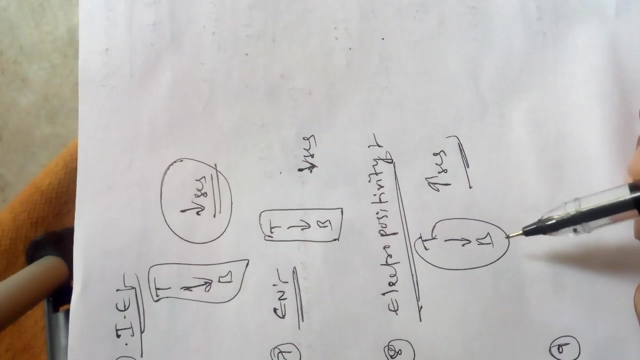 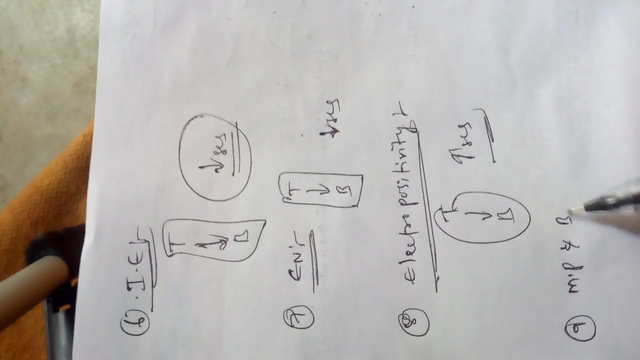 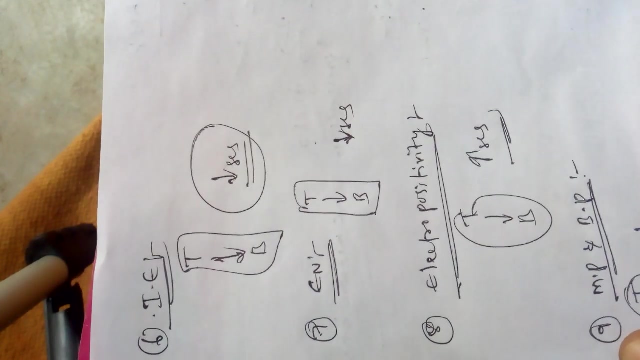 a electro positivity, uh, electro positivity, what happens top to bottom, definitely increases because electronegativity is here decreases definitely. electro positivity increases here. ninth property: again it is um, yes, important, that is melting point and the boiling point: what from top to bottom? what happens here, top to bottom melting point and the boiling point is: decreases, okay, only because of uh. metal metal bond strength is decreases. okay, moving down the group, what happens? metal metal bond strength is decreases? when the metal metal bond strength is decreases, what happens? definitely inter-atomic forces- inter-atomic forces are decreases- definitely. it also digs. when the inter atomic forces are decreases- definitely melting. 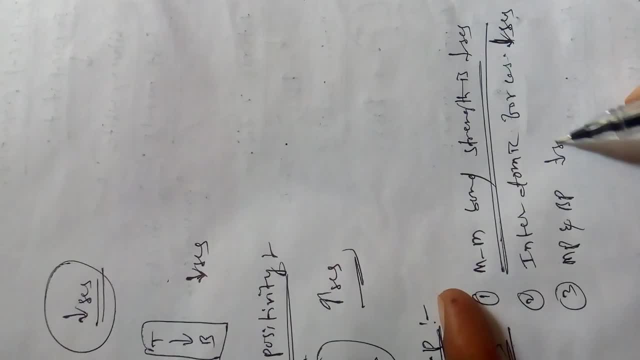 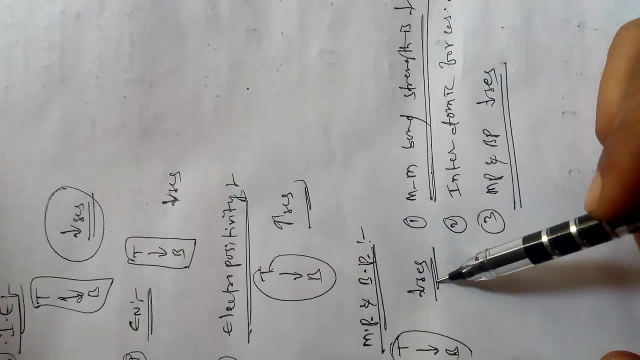 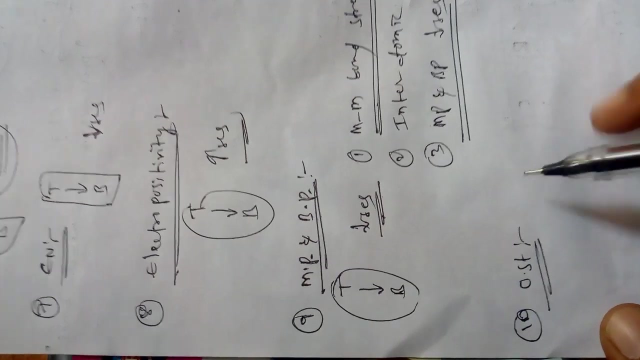 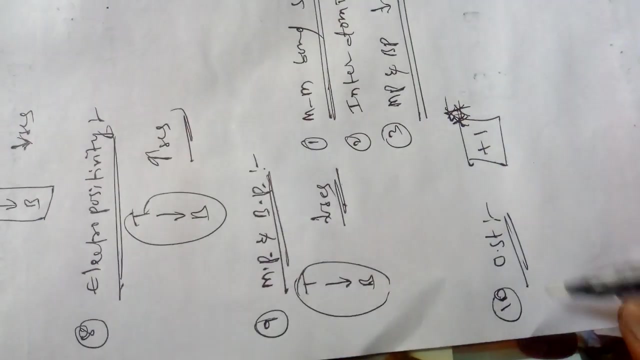 point and boiling point values also decreases, then top to bottom melting point and boiling point values are decreases, isn't it so? here a simple property, that is, tenth property, oxidation state. uh, what is the common oxidation state of first a group elements? means like plus one. plus one is a common oxidation state of first a group elements. and the 11th property: 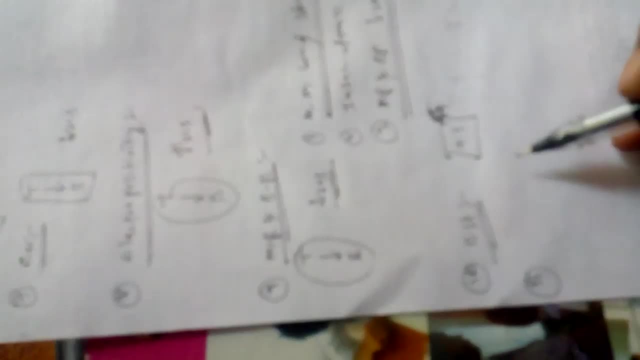 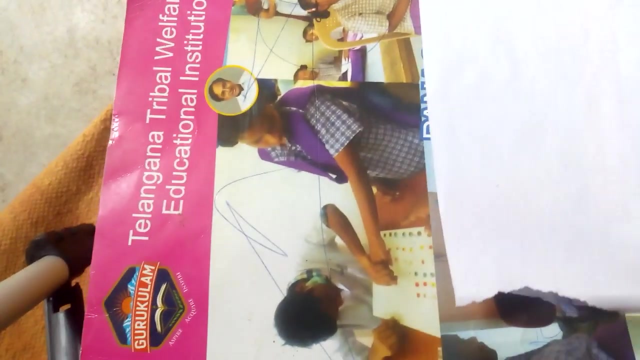 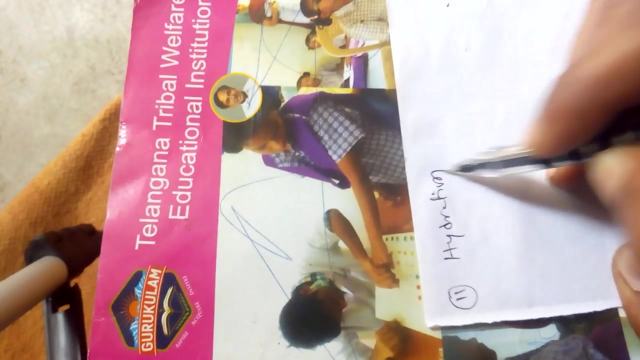 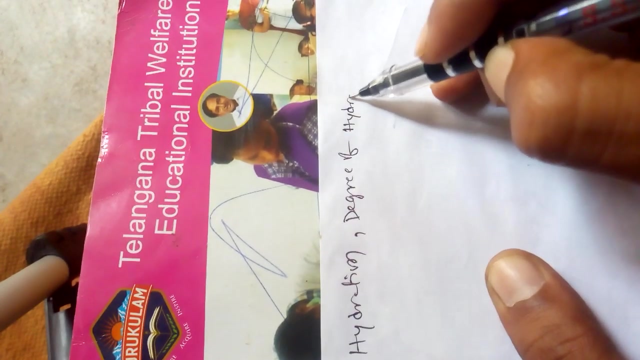 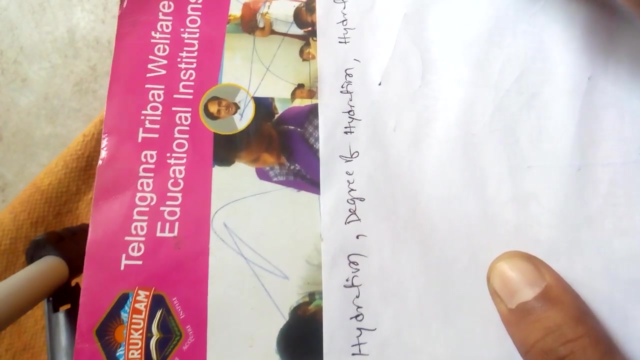 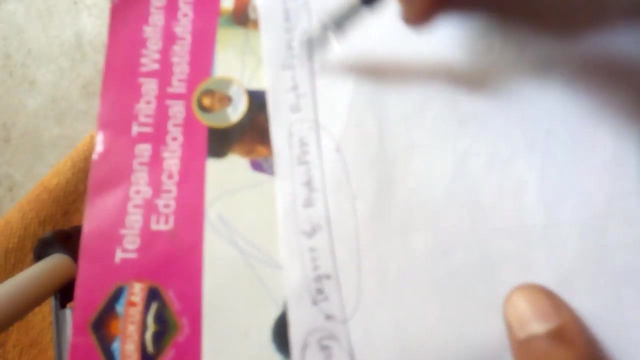 that is a important property. um is like hydration and degree of hydration and hydration energy. 11th property is very, very important. that is hydration, degree of hydration and hydration energy, isn't it? so what's the meaning of hydration? what's the meaning of degree of hydration? what's the meaning of hydration energy? okay, these are interrelated. factors. uh, actually, um, uh, in conical plus or weasel, uh, if you taken uh aqueous solutions. okay, this is a aqueous solution. when alkali metal is placed in this aqueous solution, definitely spontaneously. what happens? it? alkali metal undergoes ionization. it forms metal cation. 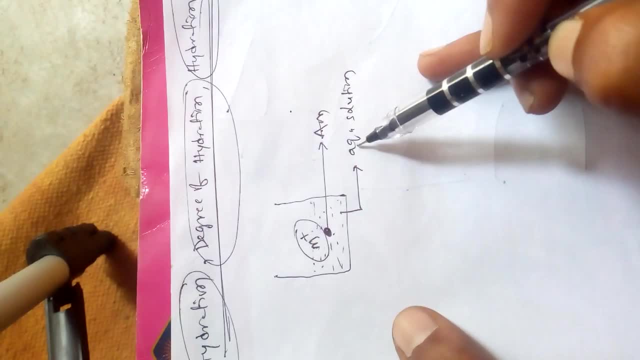 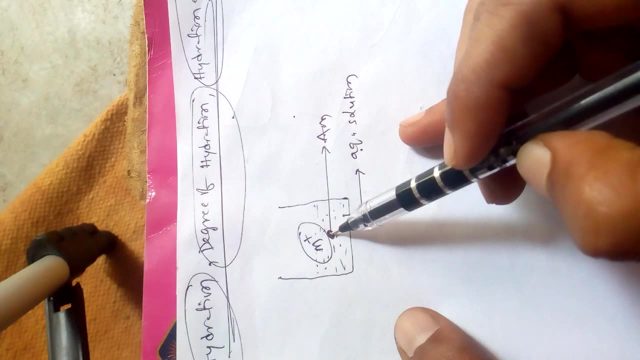 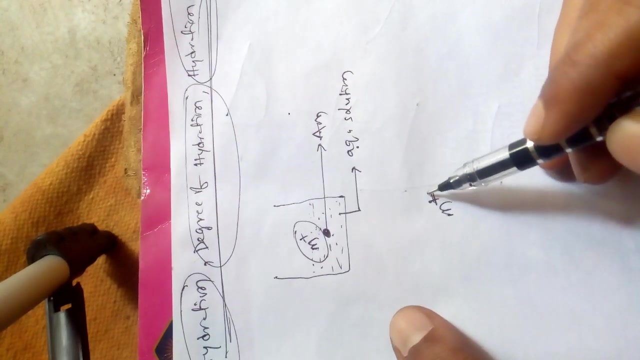 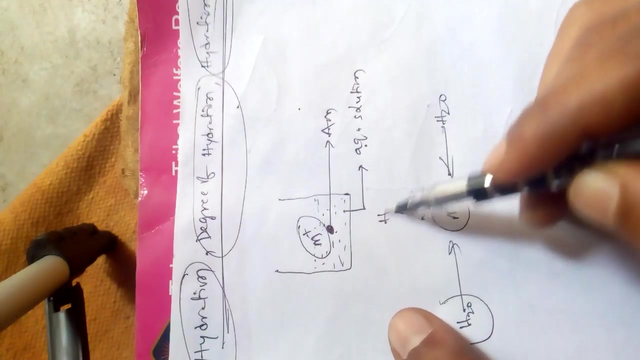 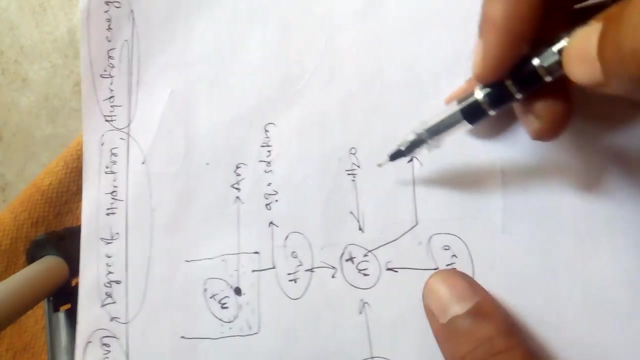 okay when the alkali metal is placed in aqueous solution spontaneously. these are. these are alkali metal undergoes ionization forms metal cation which is surrounded by polar water molecules. this metal cation is surrounded by polar water molecules, isn't it so? here, this surrounded metal cation is known as hydrated ion. what's the meaning of hydrated ion? 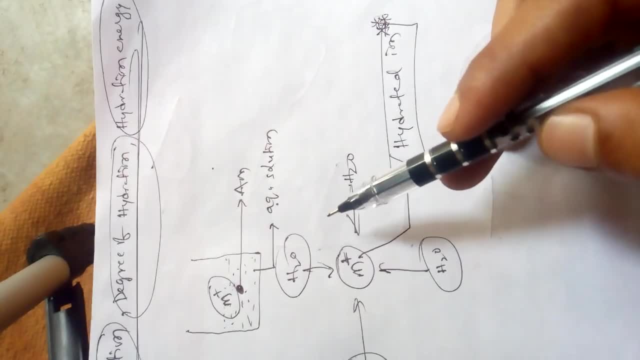 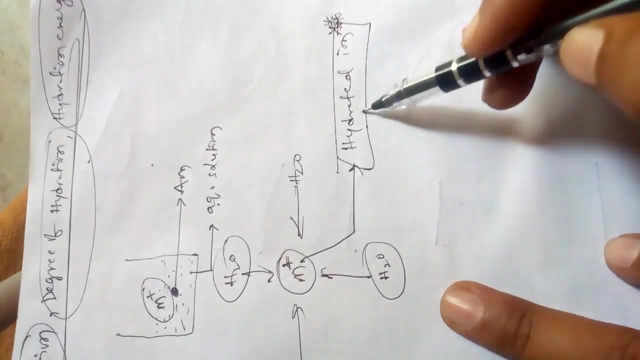 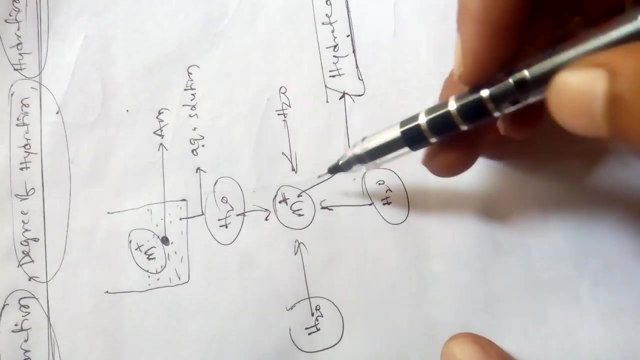 the metal atom, the metal cation, which is surrounded by polar water molecules. this cation, this cation is this. this cation is known as hydrated ion. okay, these phenomena is known as hydration. okay, hydration means nothing. but here, when the atomic, when the alkali metal is placed, 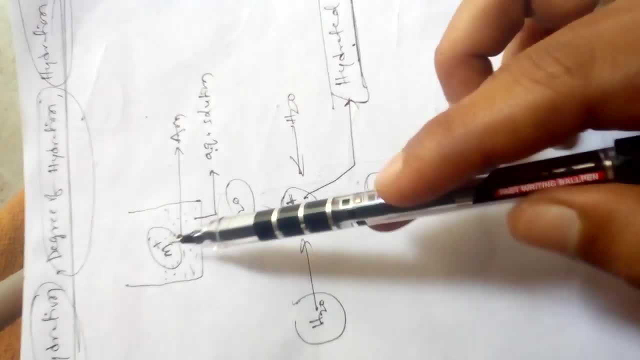 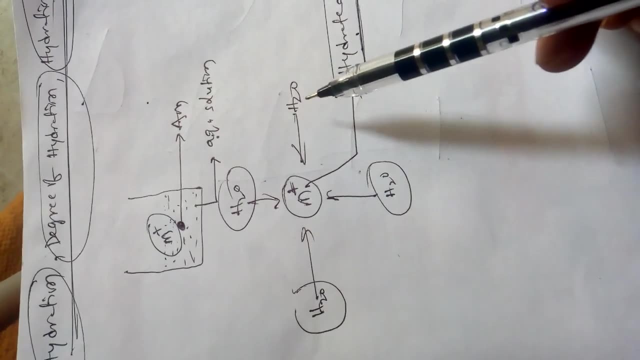 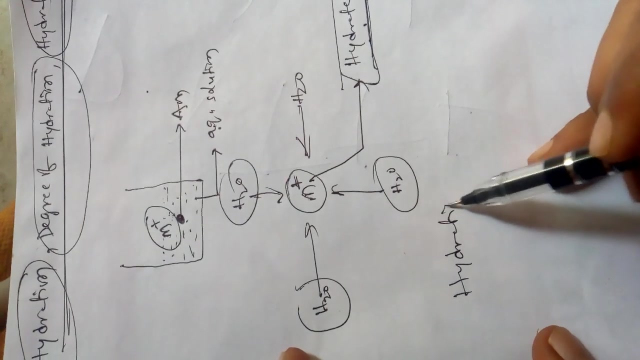 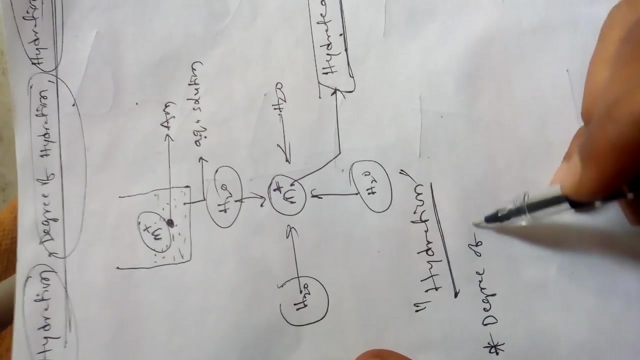 in the aqueous solution, then what happens? then? it undergoes ionization from metal cation. okay, this metal cation is surrounded by polar water molecules and it forms hydrated ion. this phenomena is known as hydration, isn't it in this hydration? just we need to know here degree of hydration. 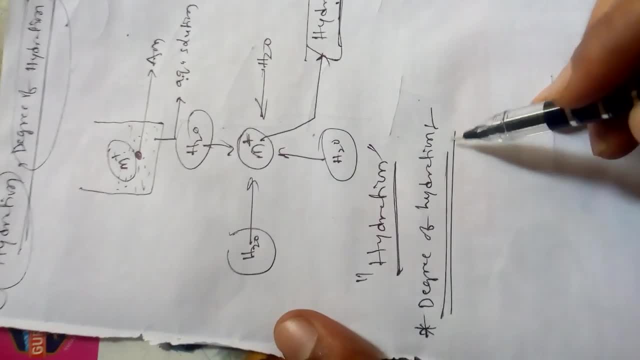 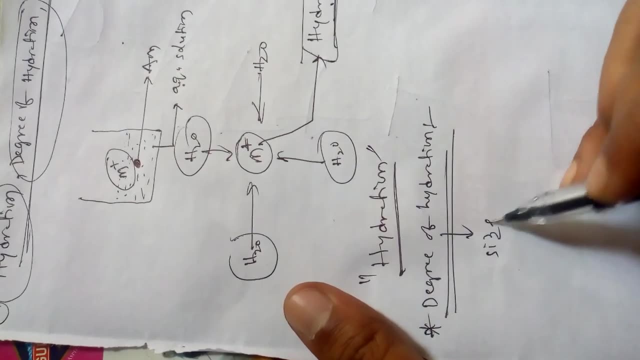 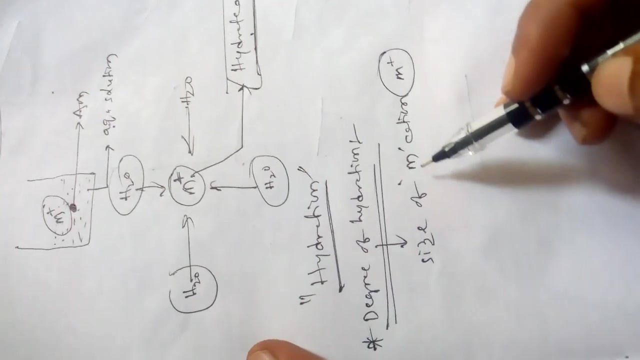 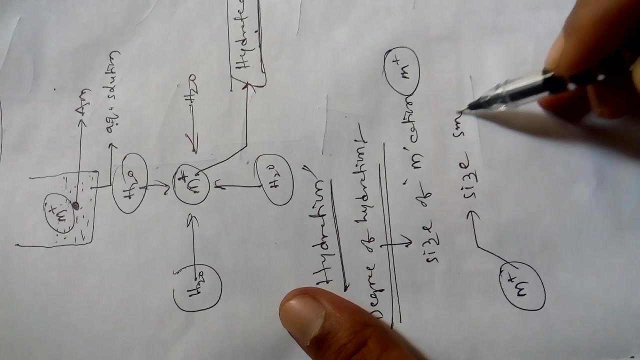 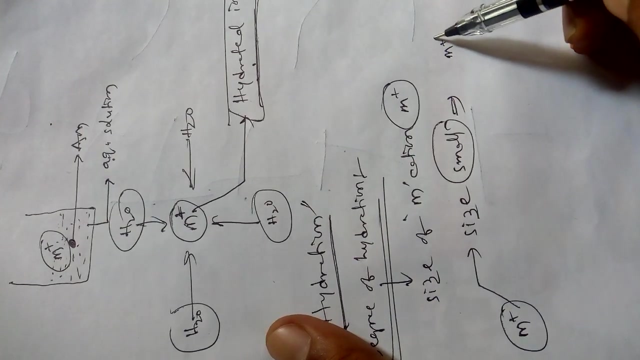 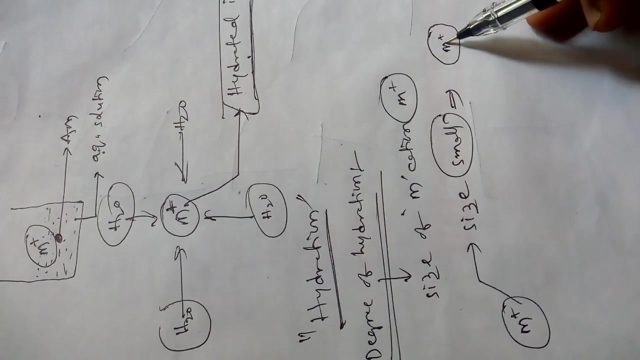 what is the meaning of degree of hydration here? the degree of hydration is depends upon size of metal cation that is emplaced. okay, if snowflakes metal cation size is small, what happens? definitely when the metal cations my size is small? this nuclear charge, this metal cation nuclear charge. is works up to almost like this, or it lid is opening the solution. so here, if the concentration of the madam jakie, which is a Quaternara ceramic, require the whales too, if Namuragram nuclear giving seizure, all the into that Gray basis Cide H, presto, okay, so this is the whole thing. you the crystal. 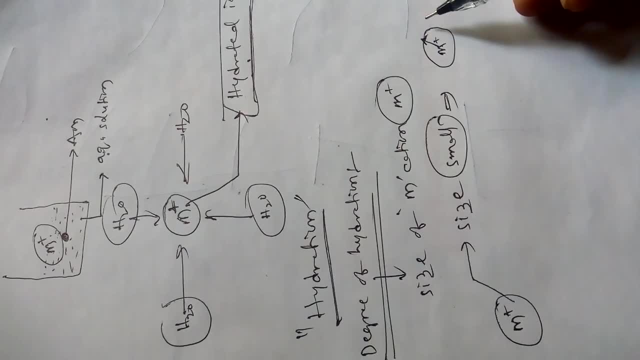 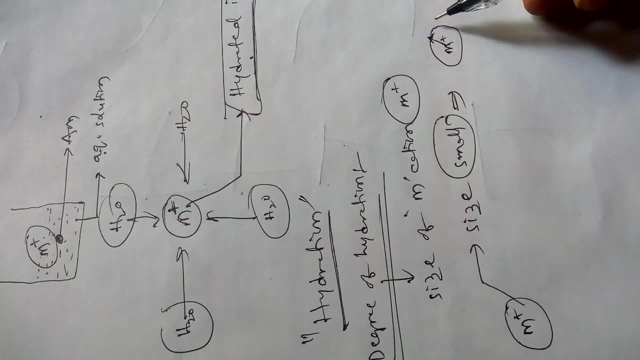 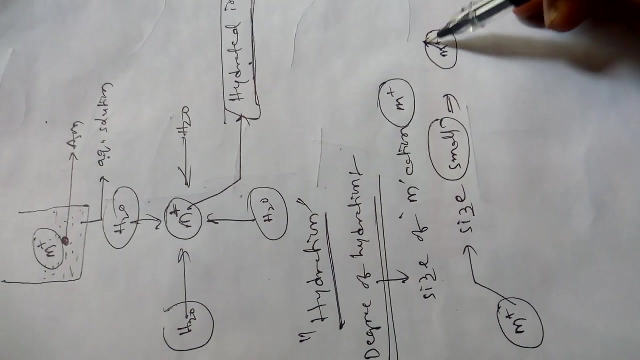 outermost energy level. okay, it means if metal cation, small in size, it nuclear charge- works up to outermost energy level, then it attracts more number of water molecules. here, when the metal cation is small in size, what happens? this metal, this nuclear charge, metal nuclear charge. 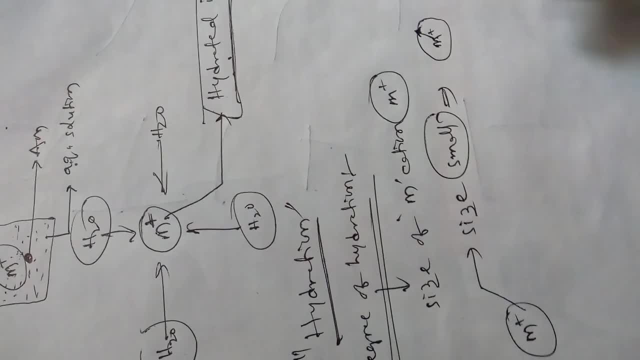 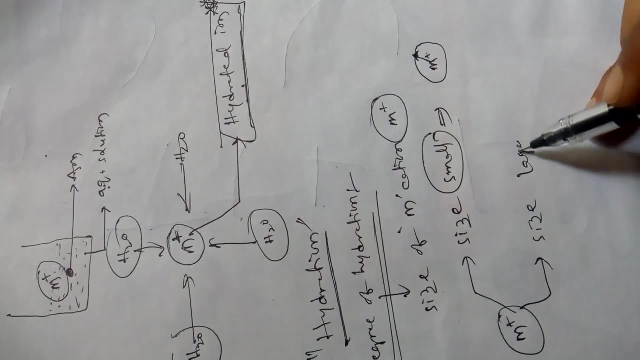 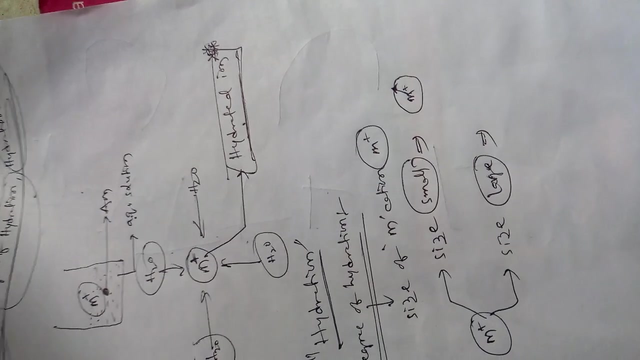 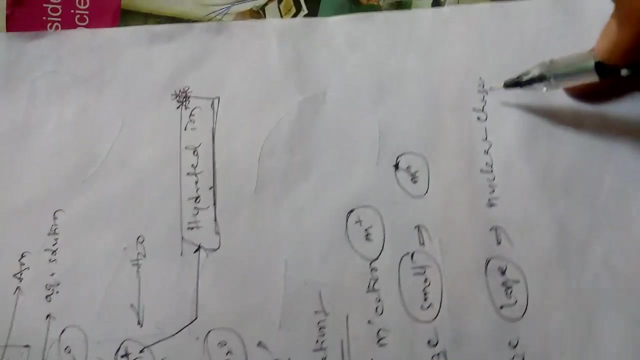 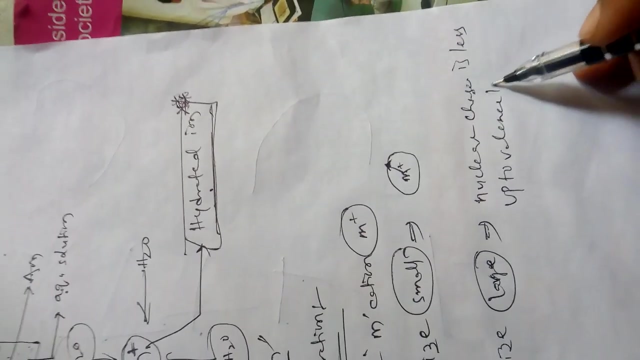 is works up to outermost energy level. so then it. then it attracts more number of water molecules easily when size is large. when size is large, what happens? vice versa, reverse, the metal cation is large, then what happens? nuclear charge. nuclear charge is nuclear charge is less up to balance. 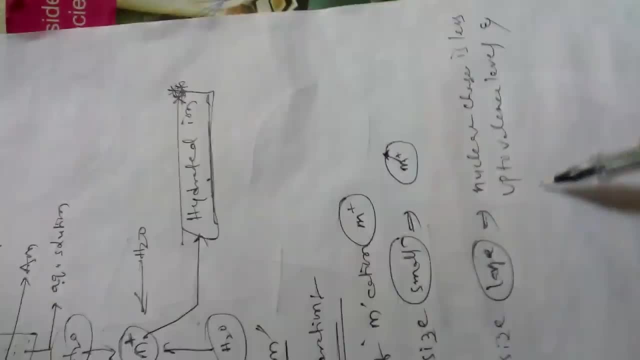 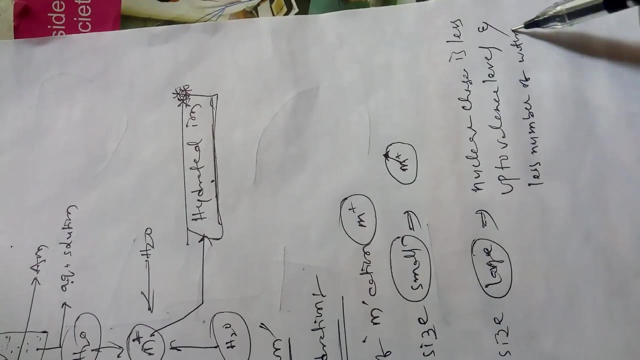 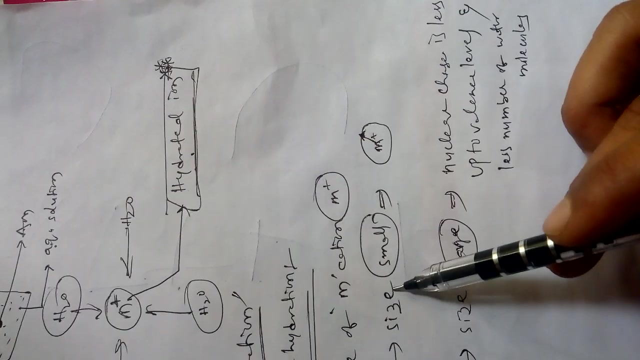 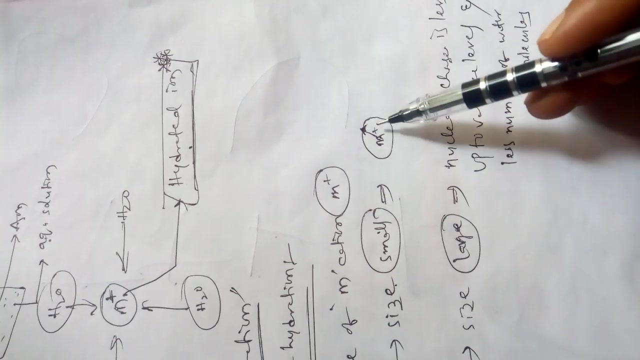 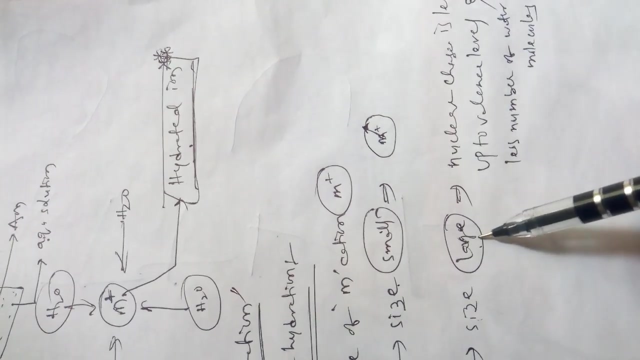 level and it attracts less number of water molecules. it attracts less number of water molecules, isn't it? if metal cation size is small, the nuclear charge is having more. when the when the nuclear charge is more, it attracts water molecules more. when the metal size is large, the nuclear charge is less. up to balance. 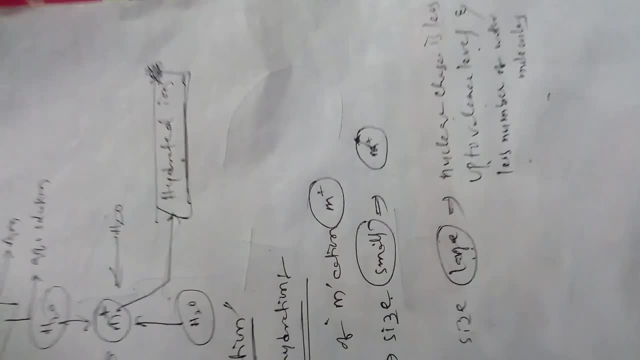 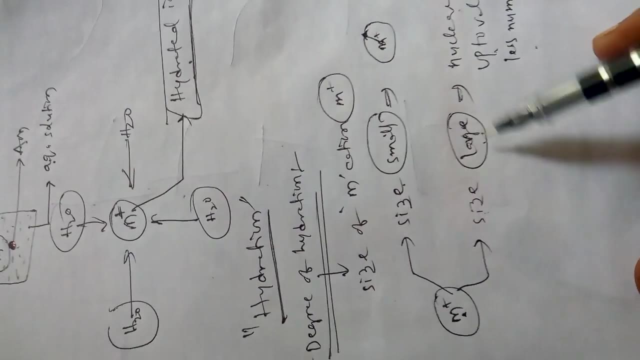 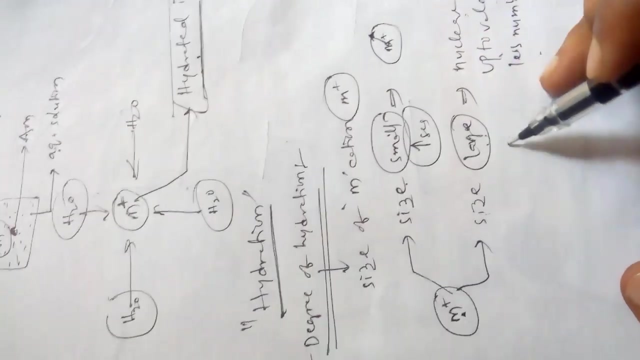 it attracts less number of water molecules. so if smile is small, a if size is small, what happens? degree of hydration is increases. if size is large, degree of hydration is decreases. okay, if small size, degree of hydration increases, if large degree of hydration decreases, isn't it so? 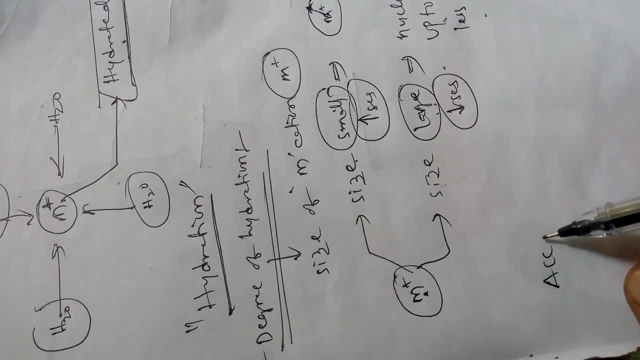 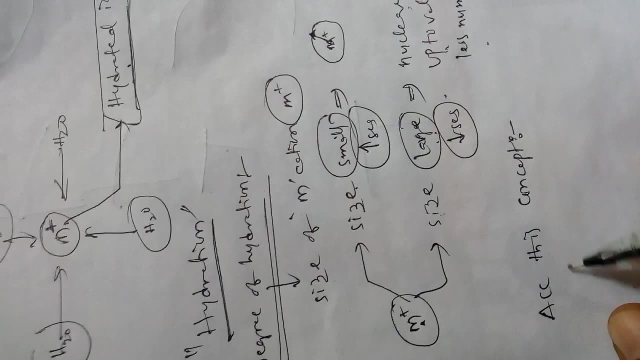 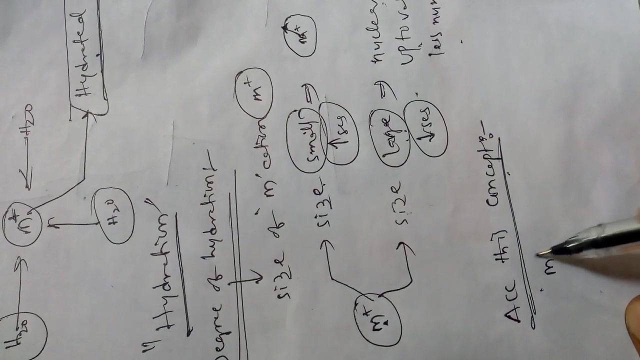 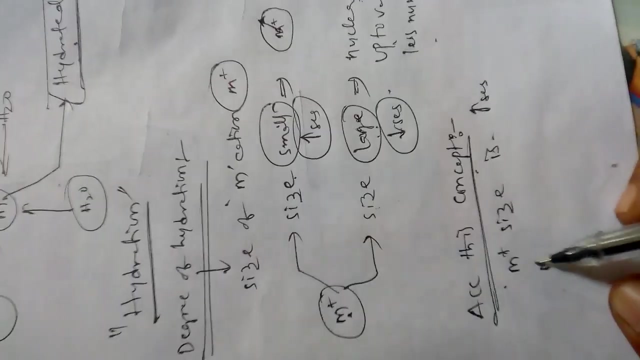 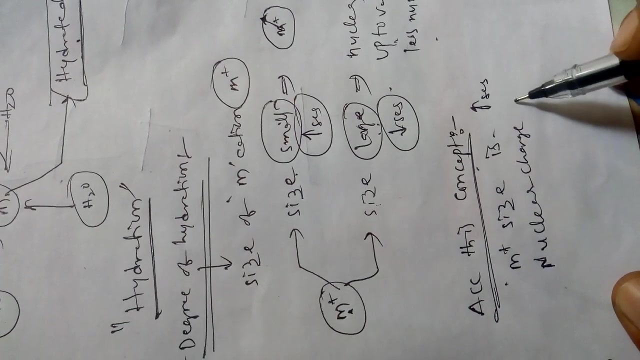 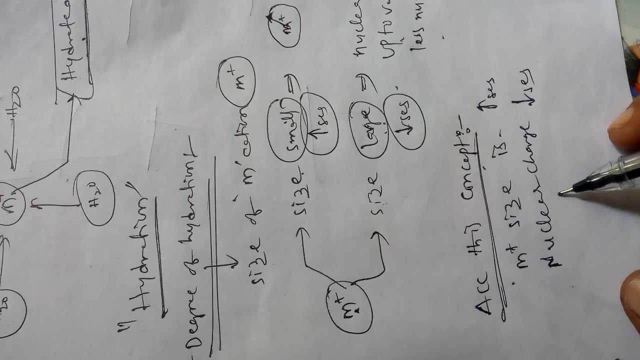 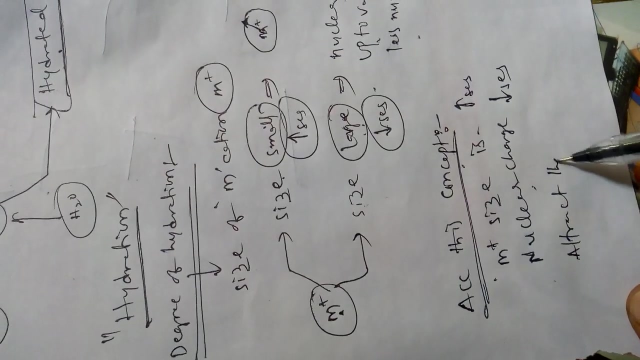 actually are you able to understanding my words? according to this concept and we are able to find out, like, when the metal size or metal cation size is increases, what happens? nuclear charge, nuclear charge up to outermost level. what happens? decreases. okay, when the nuclear charge is decreases, what happens? the tendency to attract. attract the water. 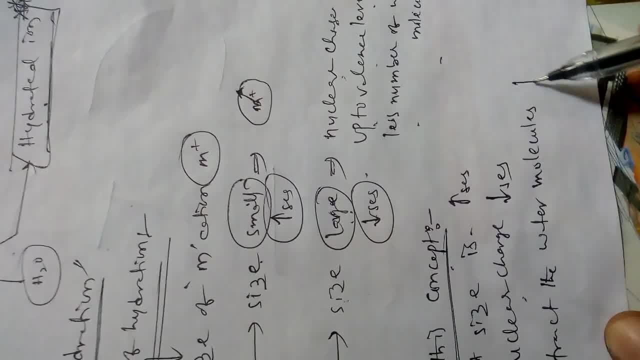 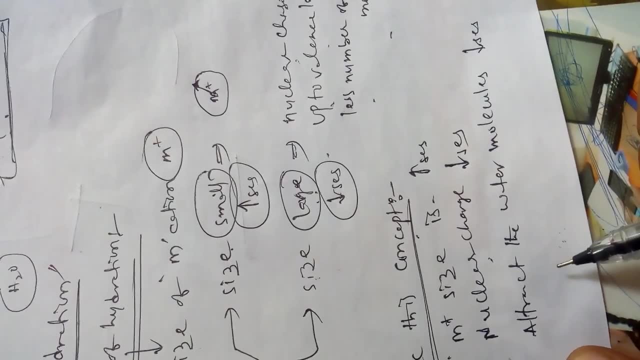 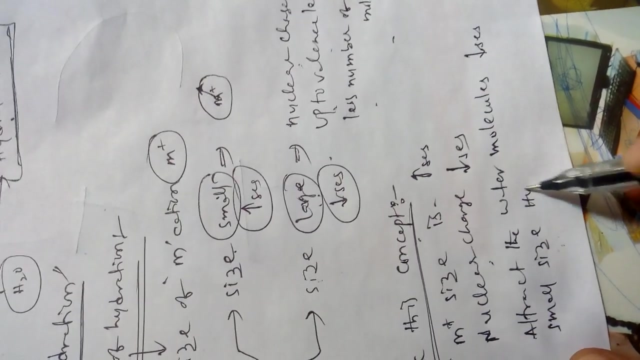 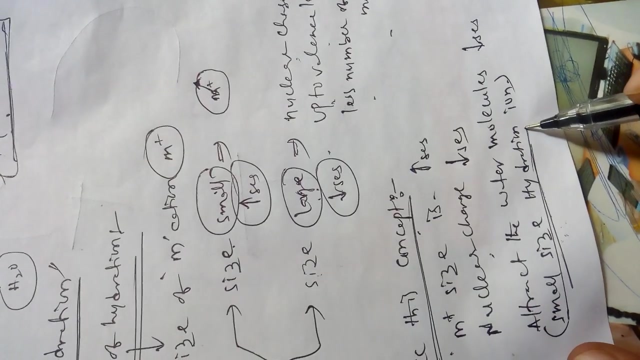 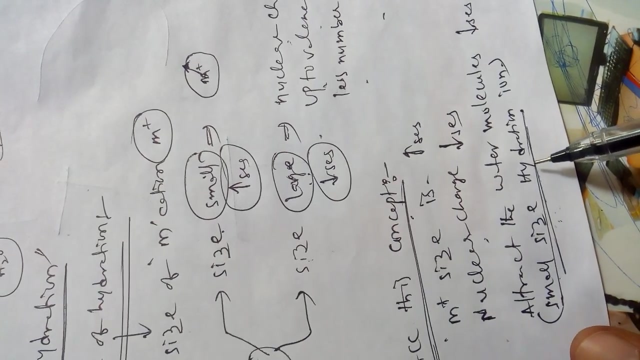 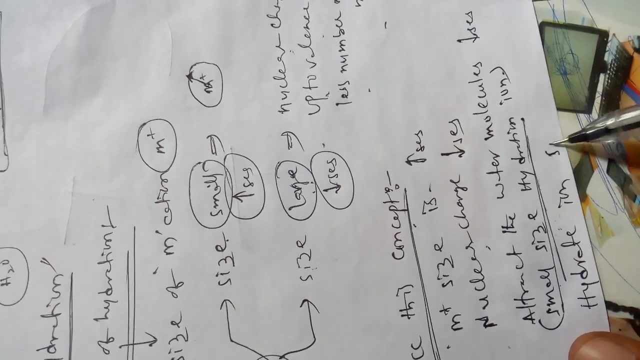 molecules decreases. definitely, when the nuclear charge decreases, tendency to attack the water molecules also decreases. then what happens here? it forms small size higher hydration ion, isn't it? it forms small size hydration ion. it forms small size hydration ion and hydrated ion. it means this hydrate ion size is decreases. hydrate ion size is decreases. okay, when the hydrate ion size is decreases. what happened? DEGREE OF HYDRATION, ALSO degree of hydration also definitely decreases. when the degree of hydration is decreases, hydration energy also decreases. okay, what the meaning of hydration energy means here? weather? When it is degree of hydration takes place during this phenomena, it releases some kind of energy. Like the amount of energy which is released during hydration phenomena is known as hydration energy. 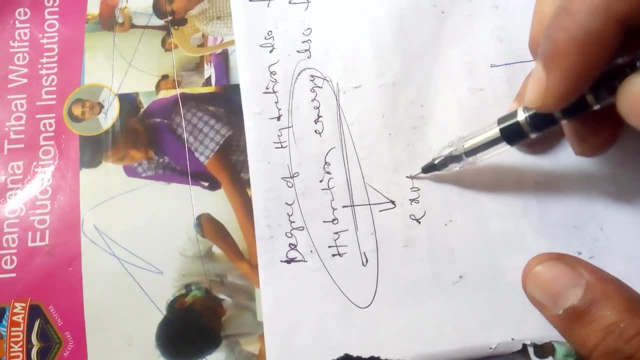 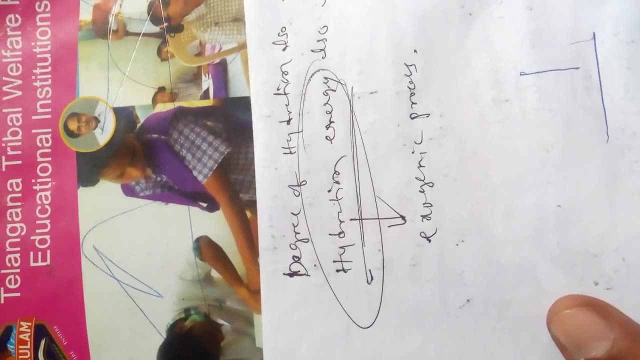 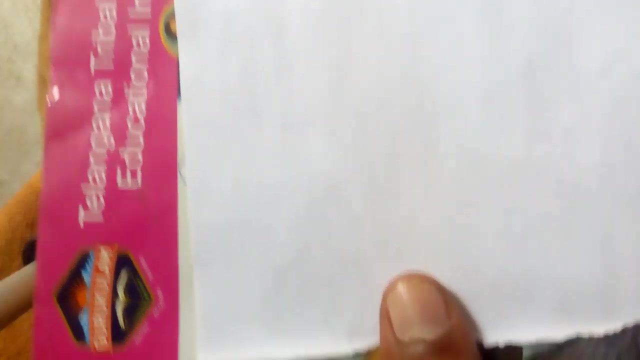 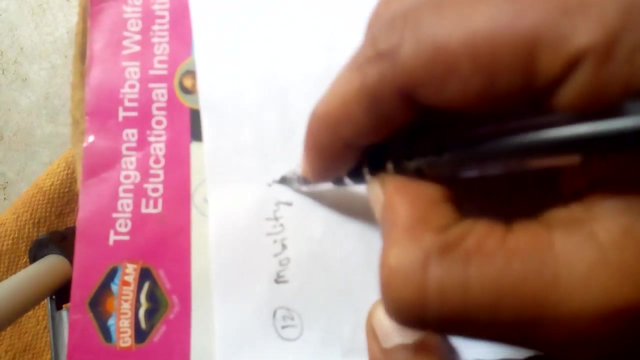 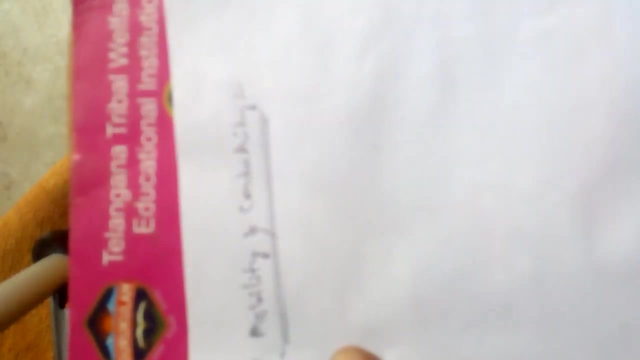 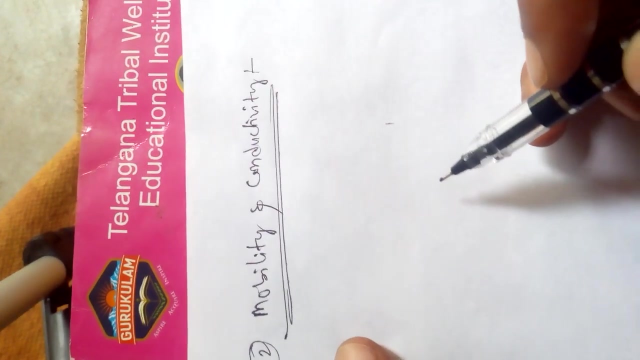 So this hydration is an exogenic process. This is about degree of hydration and hydration energy. And next property is like mobility and conductivity. And 12th property, that is mobility and conductivity. Mobility and conductivity: Actually, we think like when the top to bottom size is increasing, so mobility is decreases. 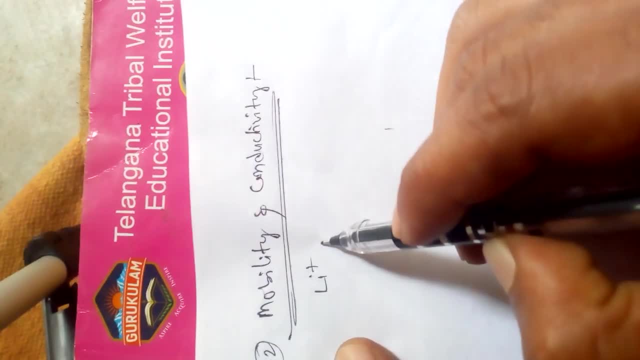 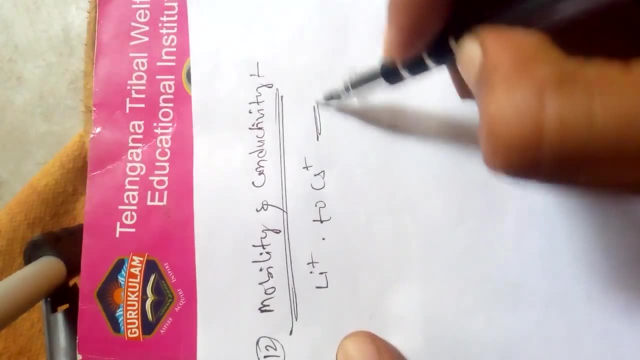 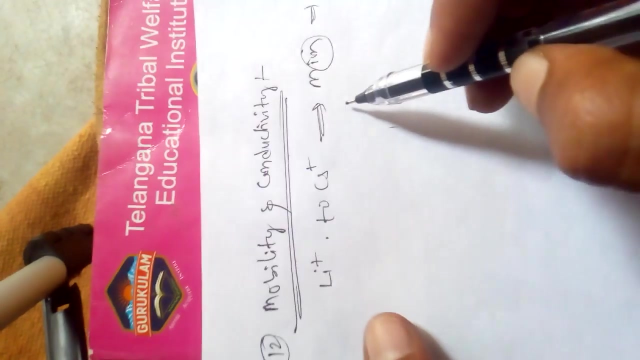 But like lithium plus to cesium, plus Lithium cation to cesium cation, As the size of metal ion, as the size of metal ion, as the size of metal ion, what happens Increases The mobility and conductivity should. 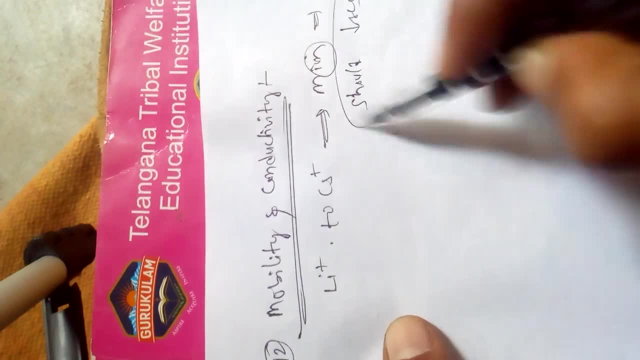 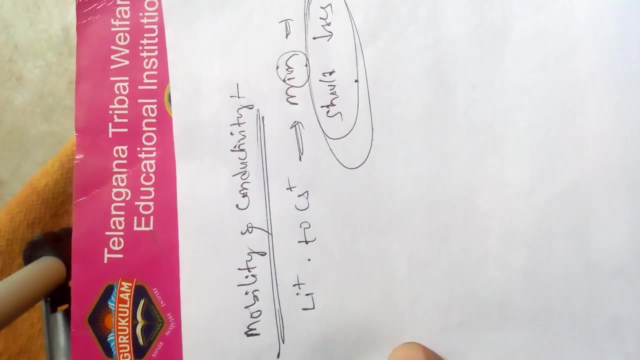 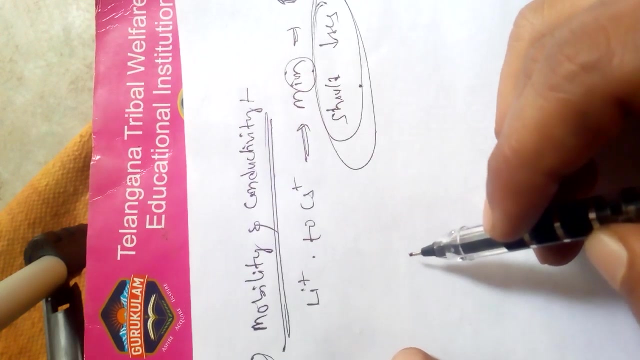 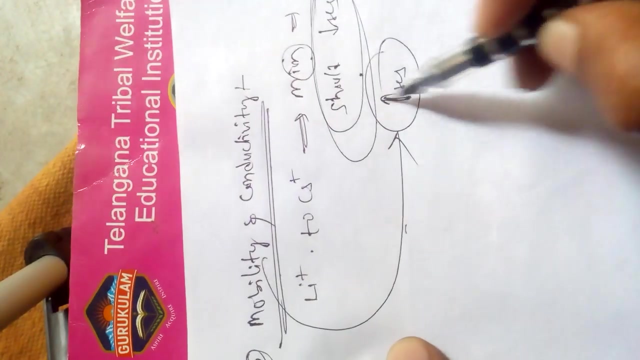 Decreases. Actually, when the metal ion size is increases, conductivity and mobility should decreases. But here, exceptions is there and the exception is like: moving down the group, mobility and conductivity is increases. Mobility and conductivity is increases, Okay, moving down the group. 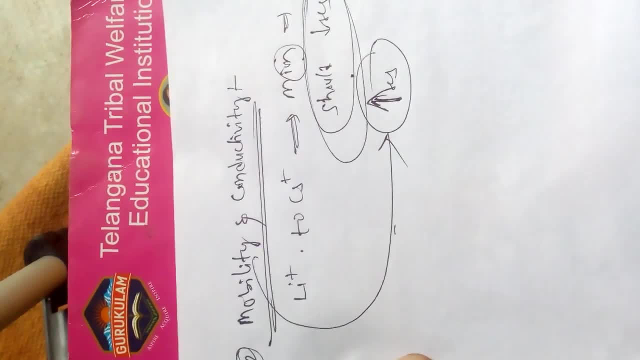 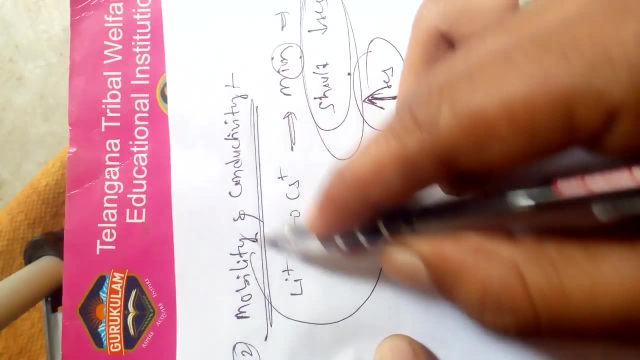 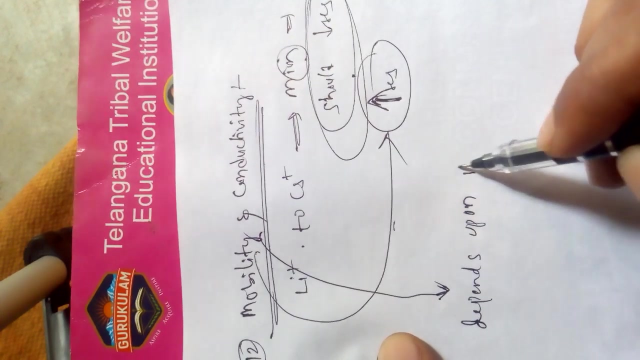 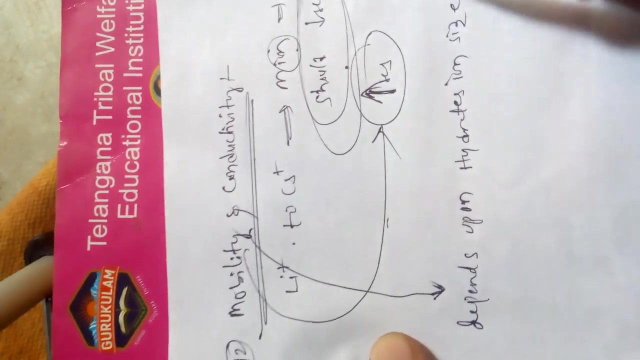 Why? because? Why, because, Actually, the mobility and conductivity is depends upon hydrated ion size. Okay, This mobility and conductivity is depends upon which factor hydrates ion size. Okay, It is depends upon hydrates ion size, Not metal cation size. Okay, 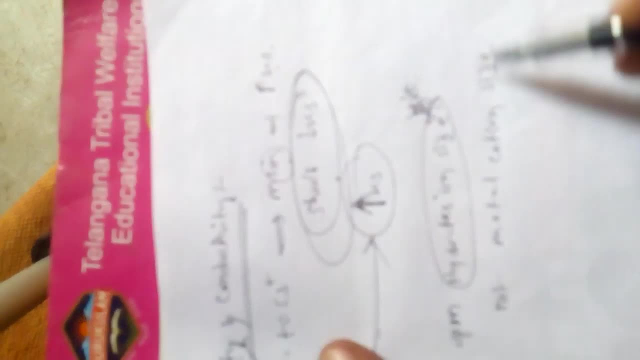 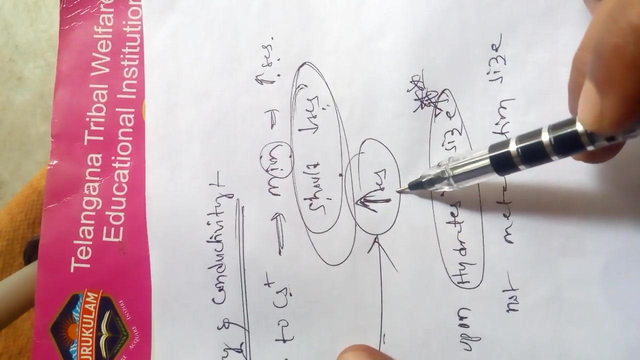 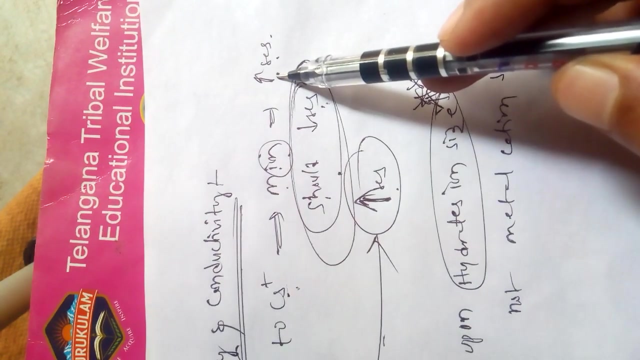 Actually we are assuming when the metal ion size is increases, it should increases, But here it is increasing. Okay, Sorry, sorry What I am saying here. lithium cation to cesium cation metal ion size is increasing, So we thought we are assuming like it should decreases, Okay. 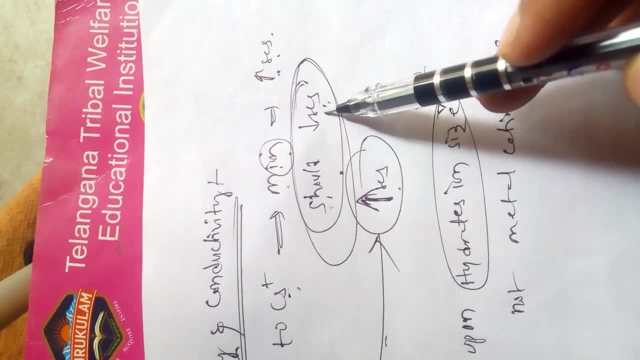 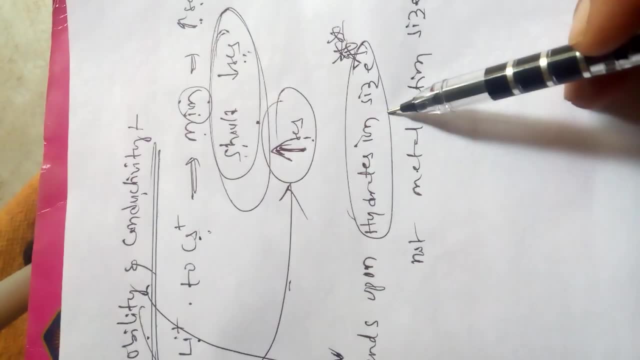 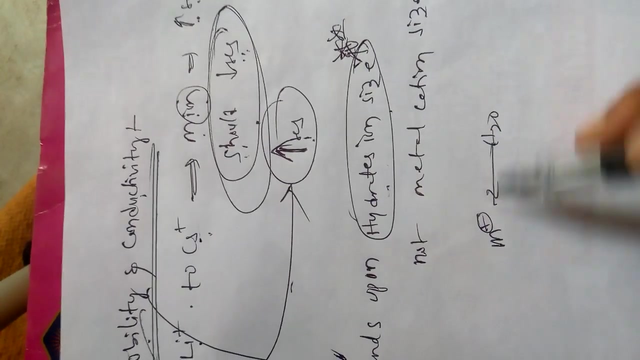 Due to weight: Okay, But here the mobility and conductivity is increasing Only because of hydrates ion size. Okay, This mobility and conductivity is depends upon hydrate ion size When the metal cation is surrounded by water molecules- Okay. 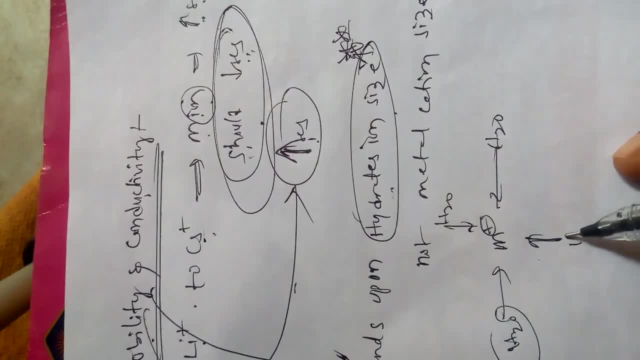 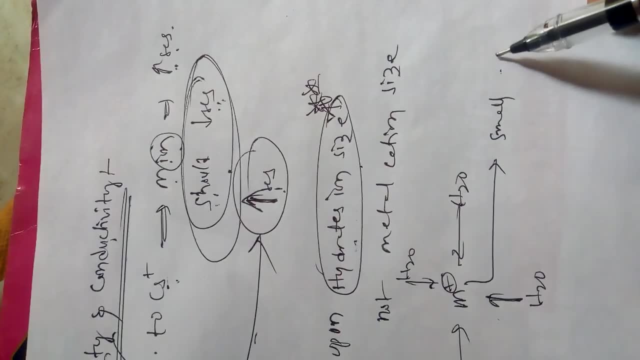 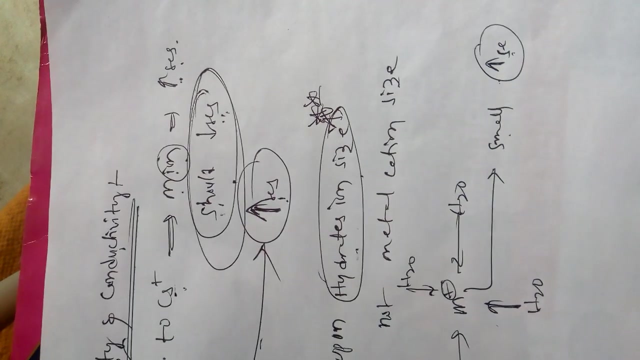 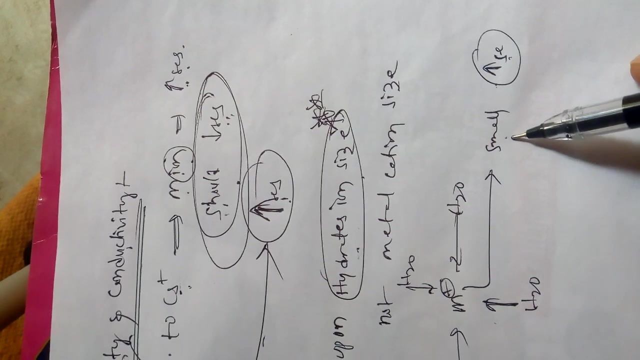 The mobility is become very tough. Okay, If small size cation is possess degree of hydration is more So when the degree of hydration is increases with respect to here Size. Okay, So small size cations are having more degree of. 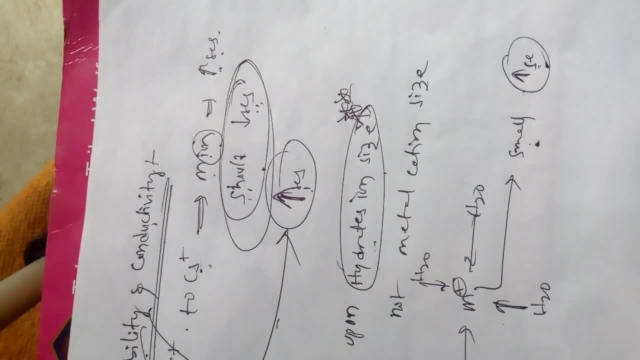 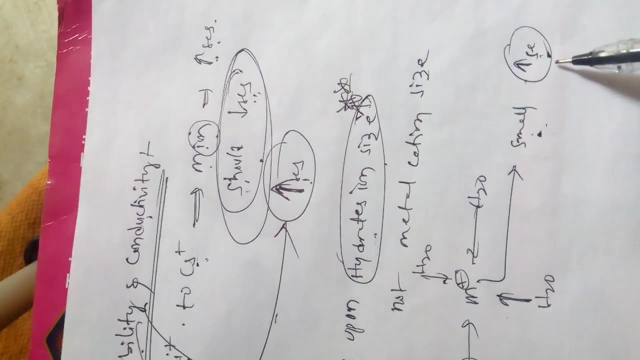 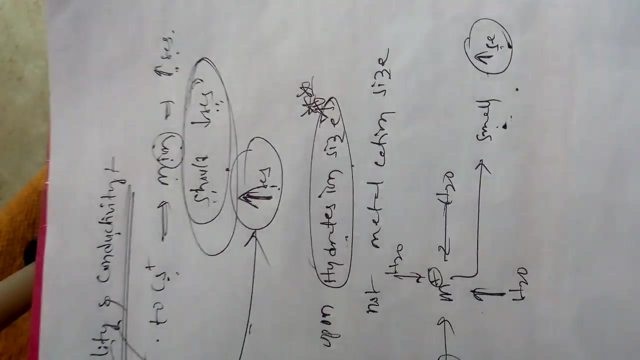 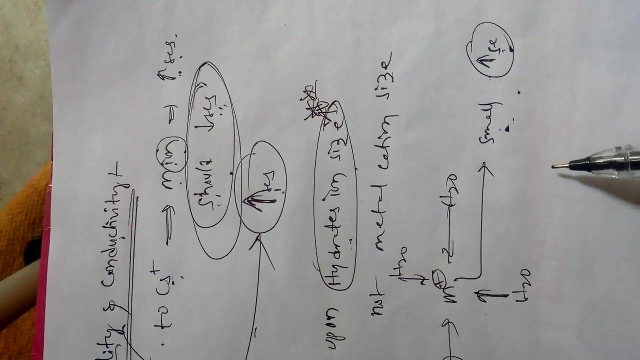 More degree of like, Like, right, Small size, having more degree of hydration energy. So it is very tough to mobile from one place to another place, So So, so. so what happening here? Moving down the group, Mobility and conductivity is increasing. 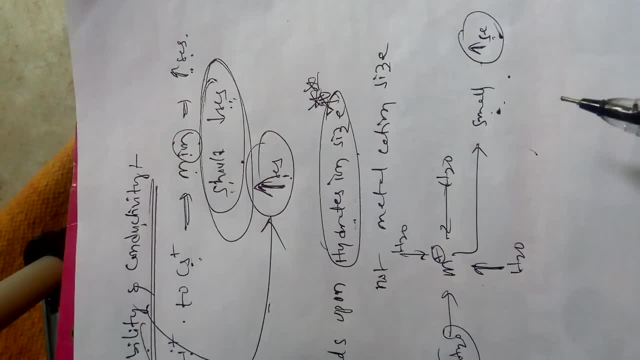 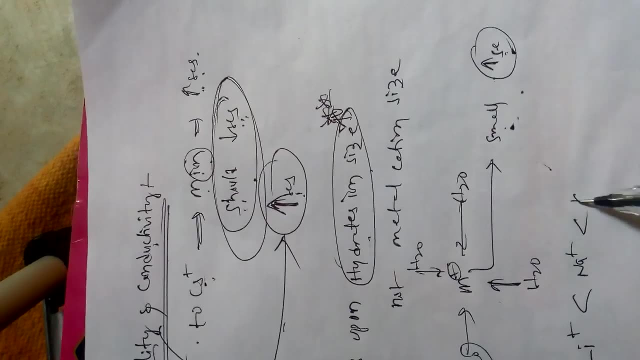 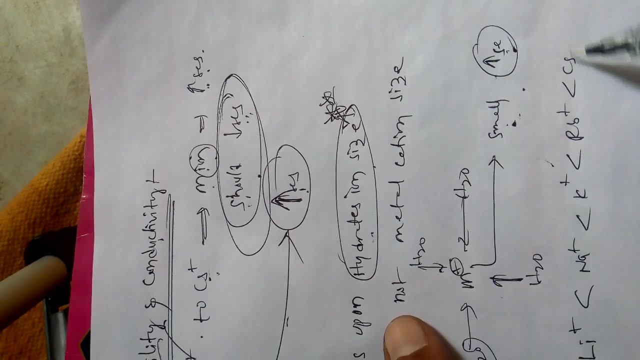 Okay, Please, are you able to understand my words? Please listen carefully. So, first of all, I am giving you order like lithium, potassium, lithium sodium, potassium rubidium, cesium. Okay, This is the order, Okay. 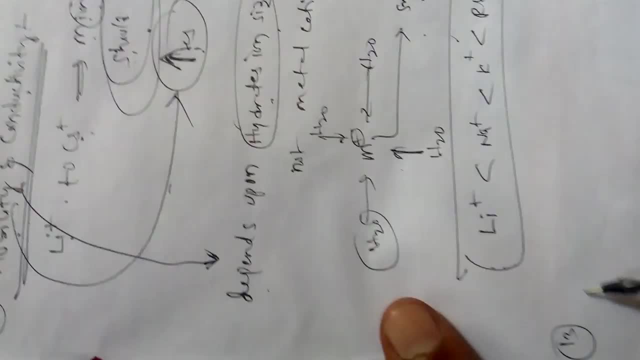 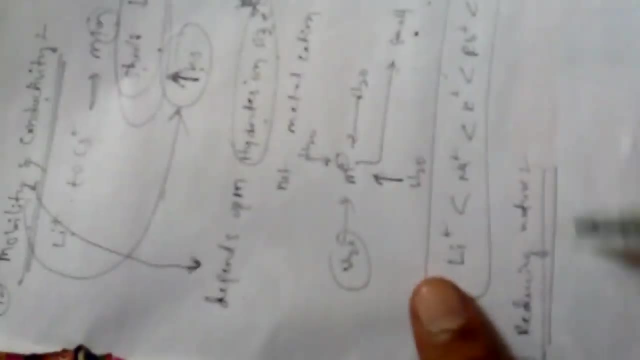 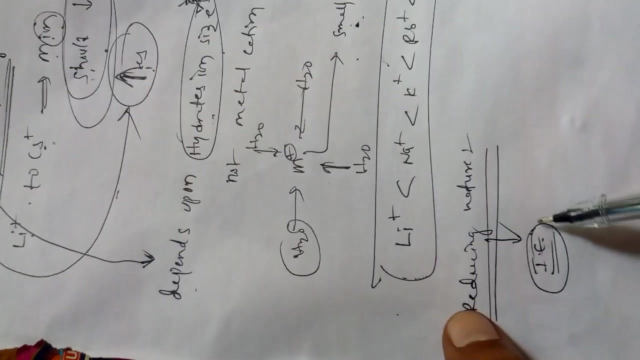 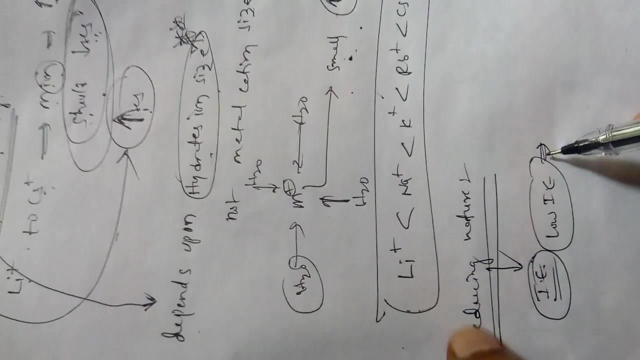 And 13 point is like reducing nature, Reducing nature. what happens actually? reducing nature of elements- depends upon ionization energy. This ionization energy, according to this element which has low ionization energy, Which has low ionization energy, It should lose electron easily. 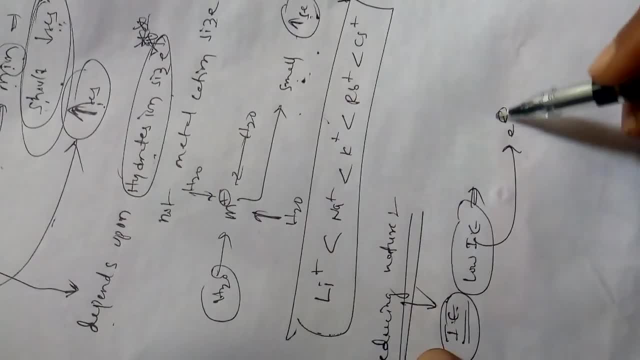 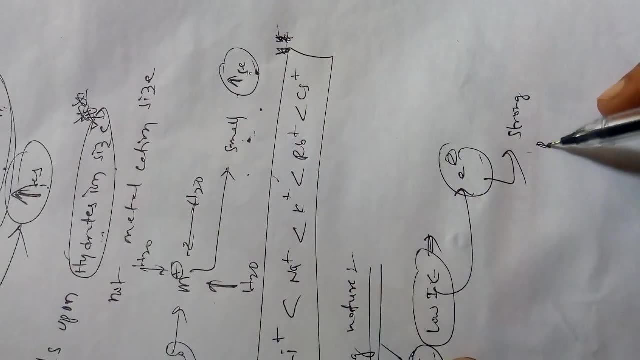 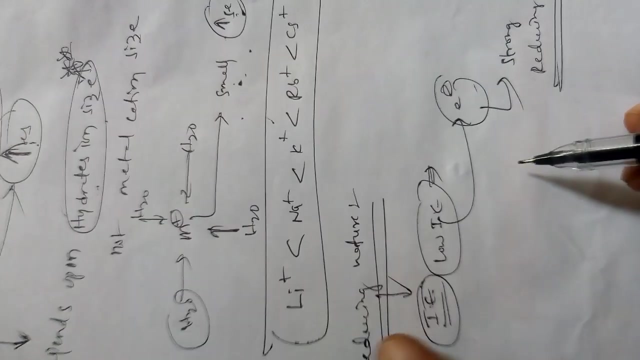 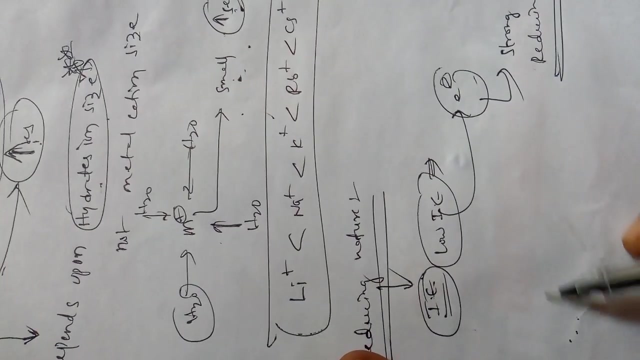 Okay, When it is lose electron easily, Then definitely it should act as a strong reducing agent. Okay, Then what happens? the moving down the group Ionization energy is decreases, So reducing nature should be increases. Okay, So moving down the group ionization energy. 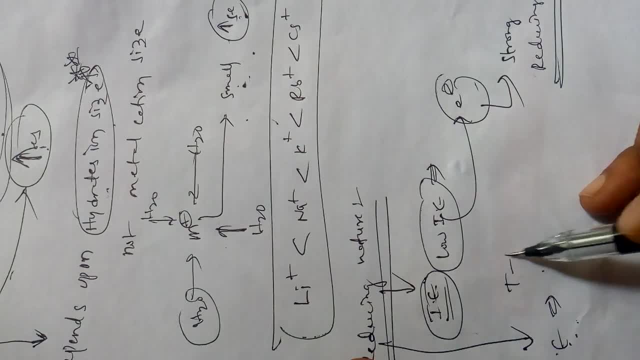 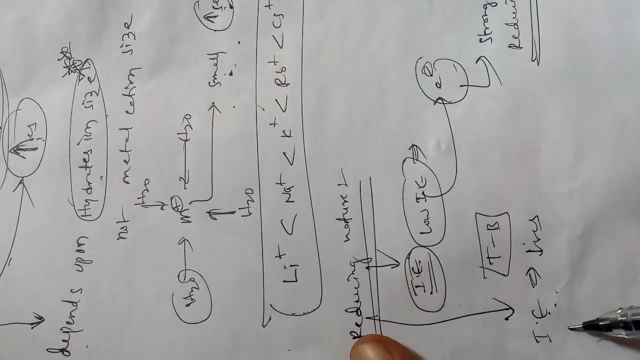 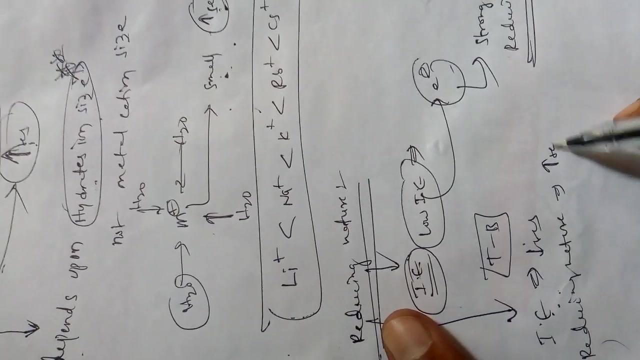 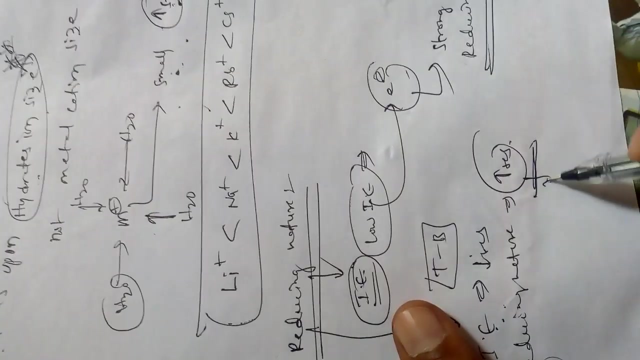 What happens top to bottom? Moving down the group. Moving down, the group Decreases. Then definitely reducing nature should be increases. Okay, Reducing nature should be increases, But here reducing nature of alkali metals is following order. Here one exception is there. Sodium, potassium, rubidium, cesium lithium. Okay, This is the exception. Okay, Why lithium act as a strong reducing agent? It is a very-very-very-very important question, And here lithium act as a strong reducing agent due to its high hydration energy. Its high lithium having high hydration energy. So by that lithium act as a more reducing nature nature and it is having a negative E naught value also and hence among all metals in periodic table also, lithium act as strong reducing agent. lithium act as 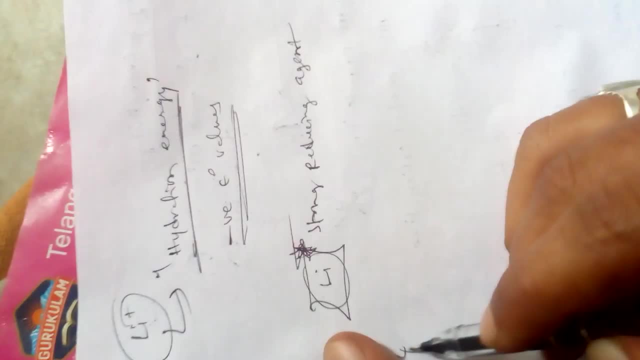 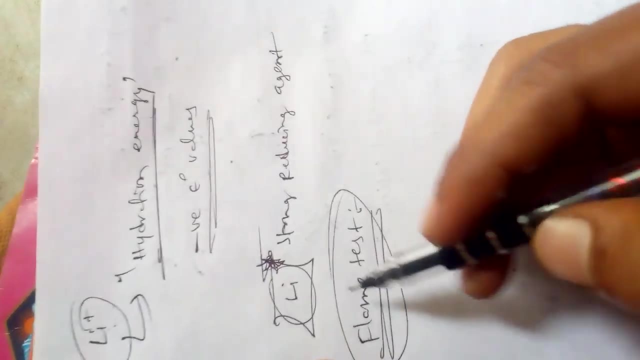 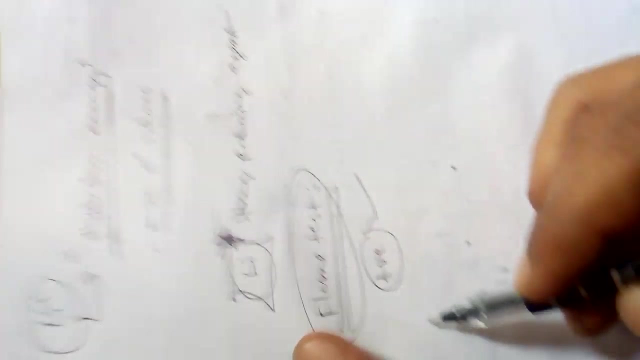 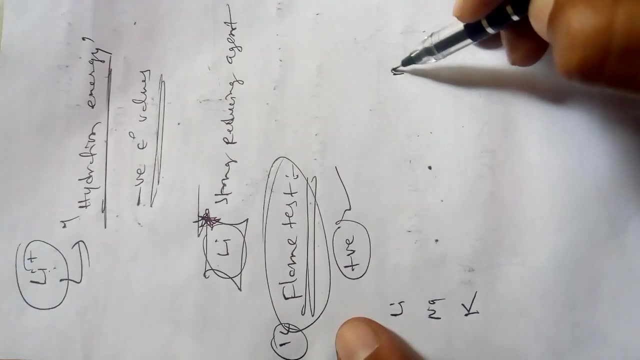 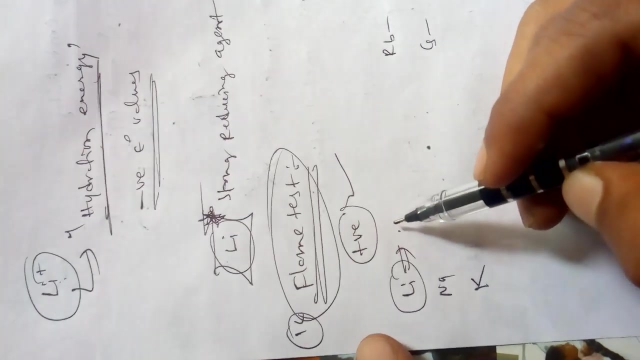 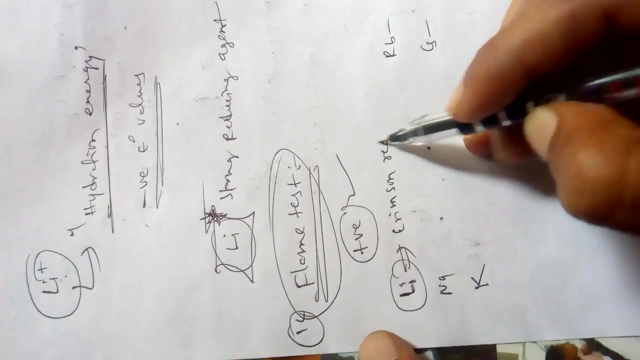 strong reducing agent. okay. and 14th one is flame test. flame test in alkali, in all alkali metals they are give positive flame test. so in that positive flame test, actually what happens in lithium, sodium, potassium, rubidium, cesium- lithium is having, when the flame test is going on, lithium is shows like crimson red color and 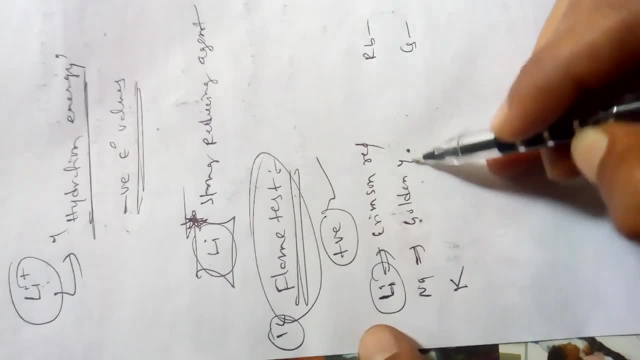 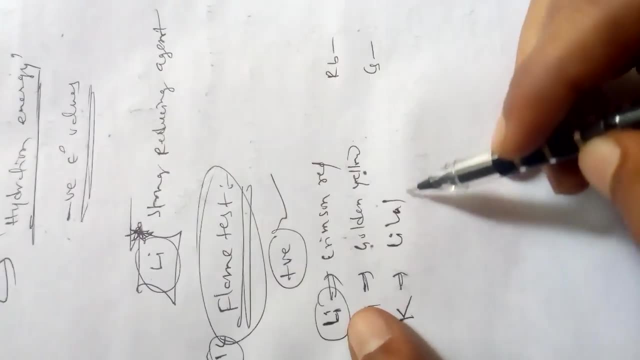 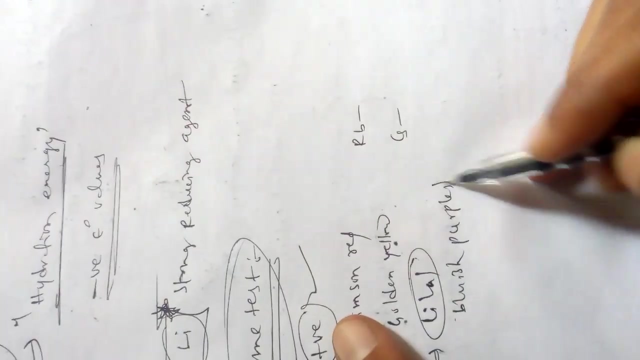 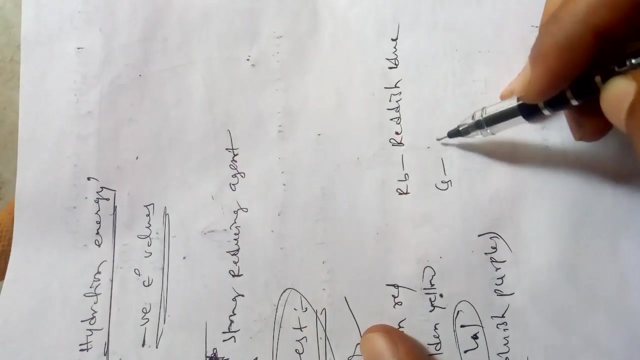 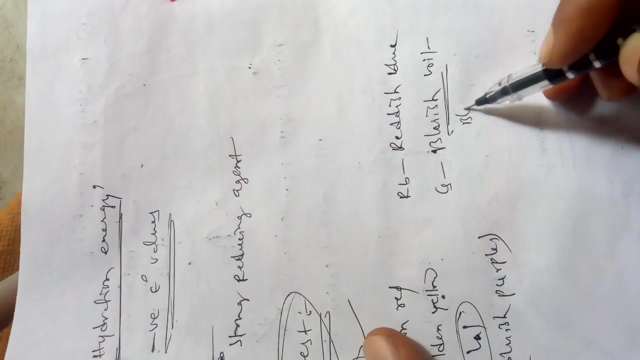 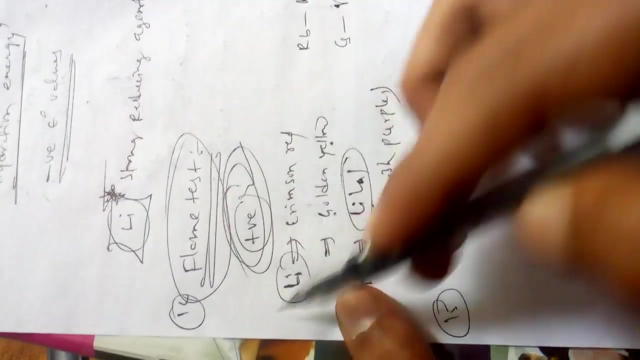 sodium having golden yellow color and potassium is like lilac. it means lilac means like bluish purple. bluish purple and rubidium is having a a reddish blue and cesium is having bluish violet. it means like blue. so first year group elements are shows positive flame test. lithium is having crimson red. 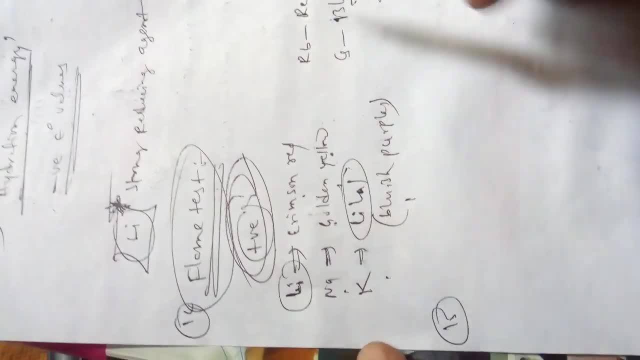 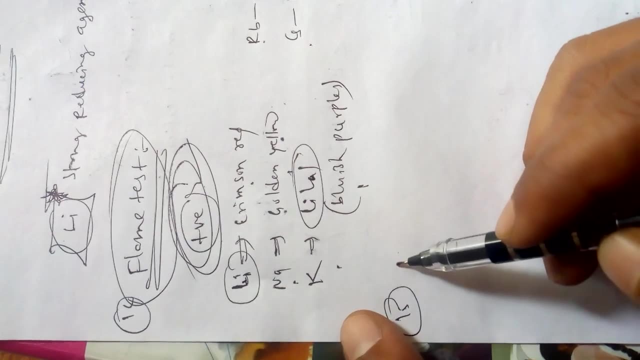 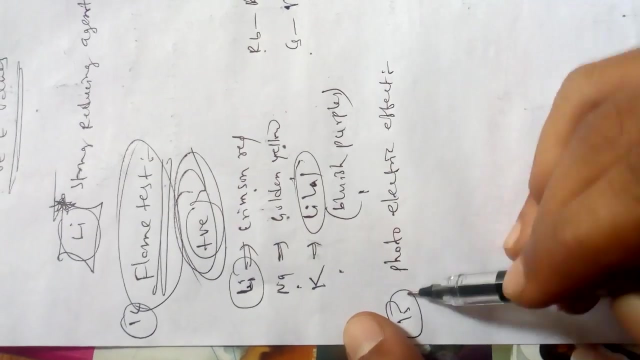 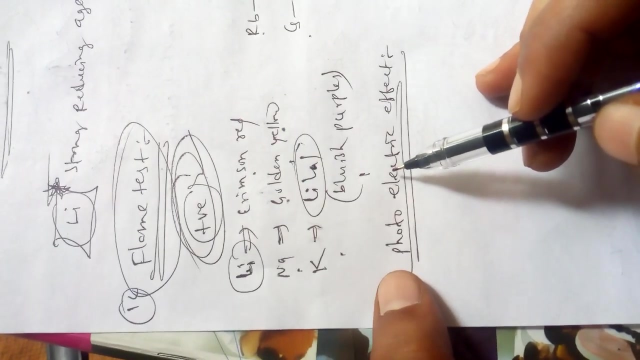 sodium is having golden yellow, potassium is having bluish, purple, rubidium is having reddish blue, cesium is having blue color. and fifth property that is, and fifth property that is important property, that is a photoelectric effect. photoelectric effect. photoelectric effect means ejection of electron of an atom in 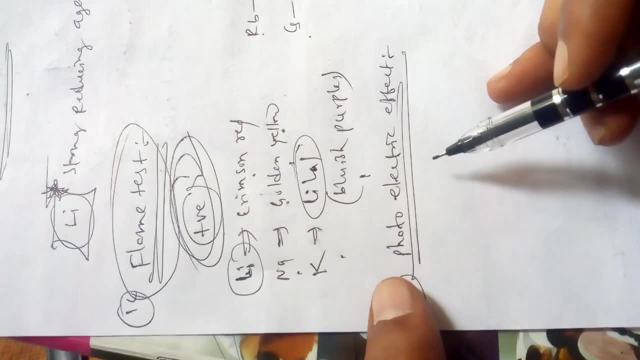 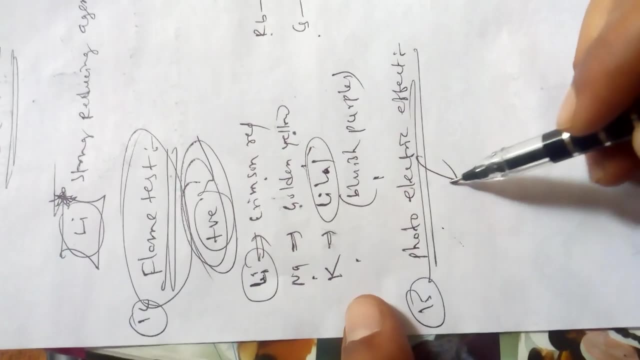 photoelectric effect. photoelectric effect means ejection of electron of an atom in the pair, right simply. but here I have doubt also one thing: photoelectric, the pair, right simply. but here I have doubt also one thing: photoelectric effect means like ejection of electrons. we know that, everyone knows, knows that. 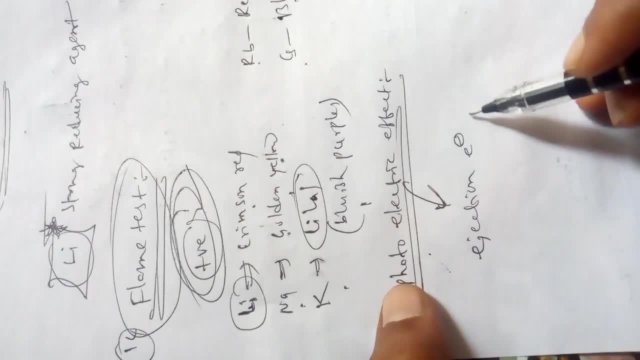 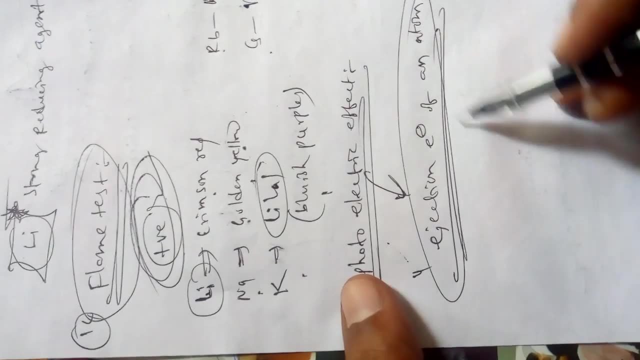 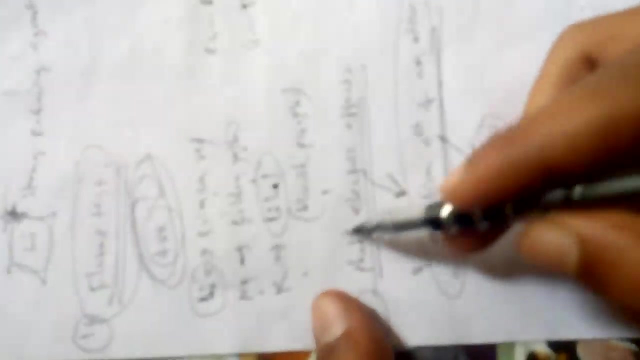 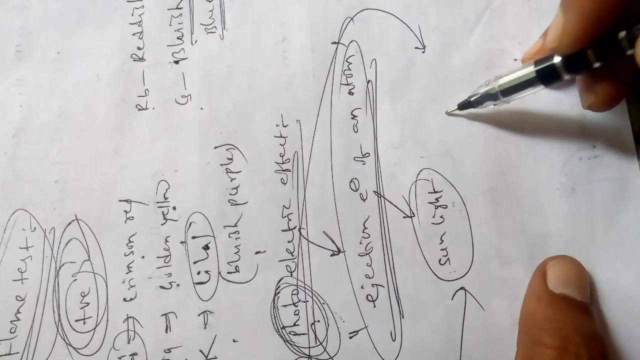 ejection of electron. ejection of electron of an atom is known as photoelectric electric. in some books they are mentioned. it is happens in presence of sunlight. okay, because of it is mentioning here photo, so it is happens because of sunlight. in some books I refer that, like in: 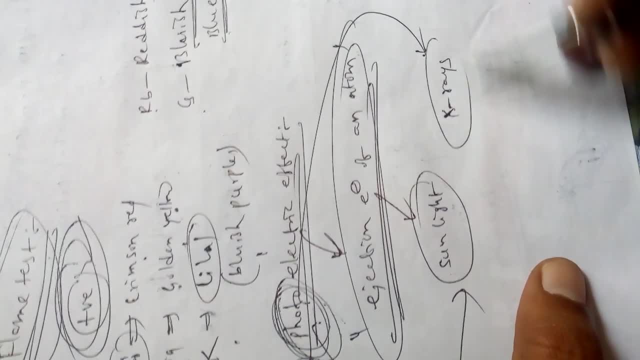 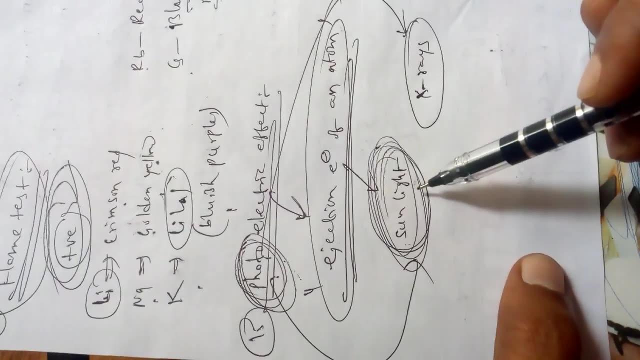 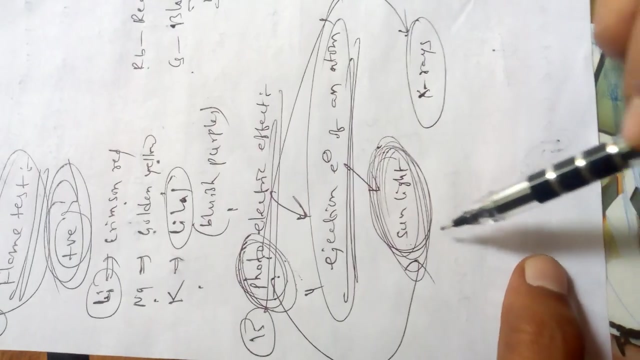 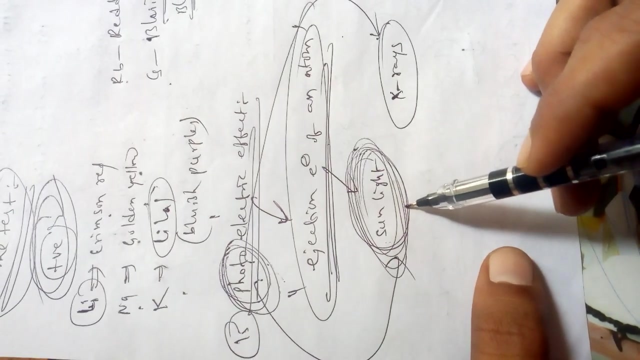 presence of x-rays. okay, it is in confusion in that actually i am major in major point of view. photoelectric effect is is the influence of sunlight. only ejection of electron of an atom in the presence of sunlight is known as let photoelectric effect. it means ejection of. 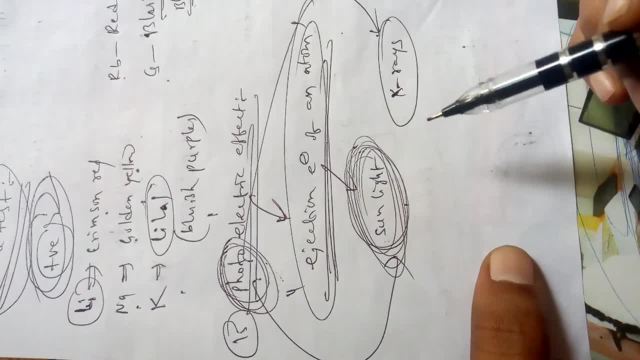 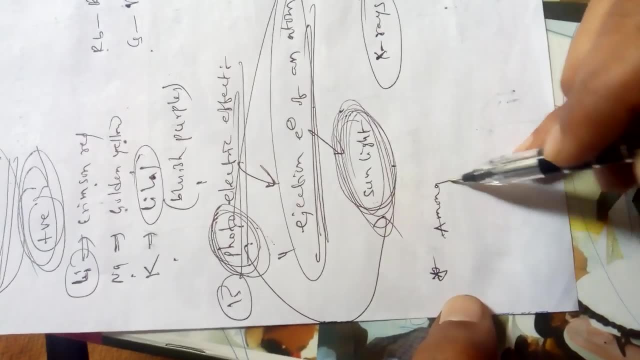 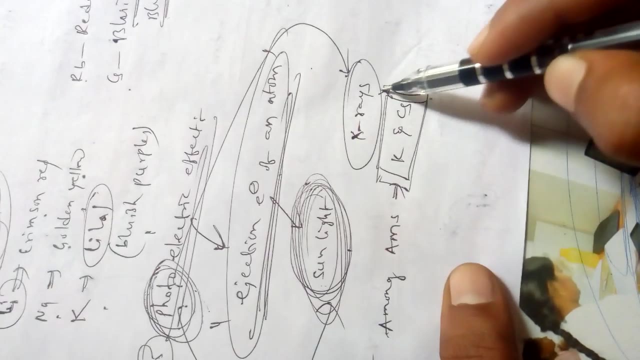 ele. ejection of electron of an atom in the presence of sunlight is called photoelectric effect. but here the entrance point of view among alkali metals, among alkali metals, here potassium and cesium. this potassium and cesium are uh. potassium and cesiums are very 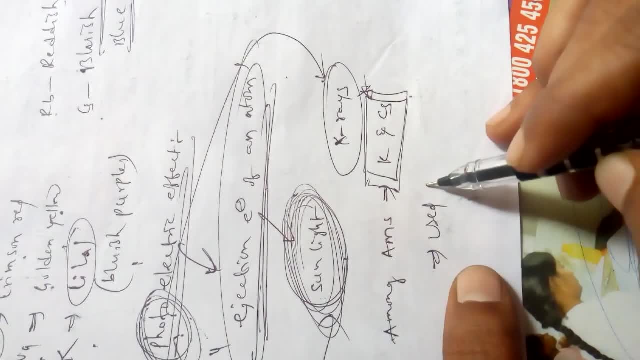 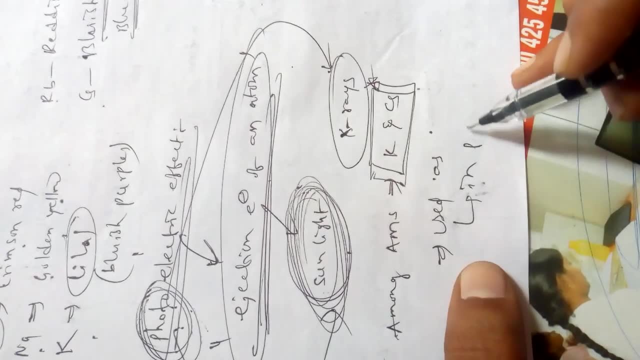 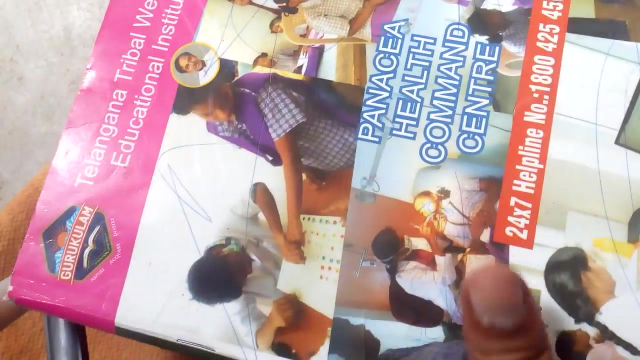 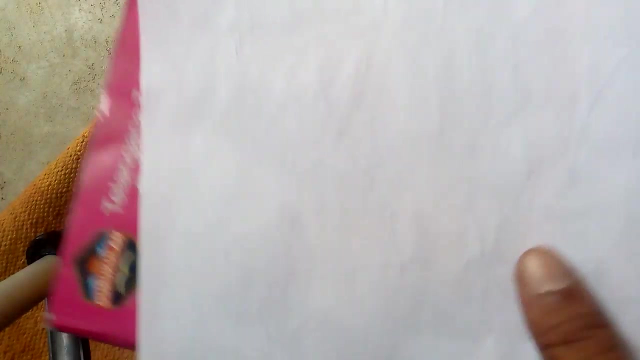 useful and a very, very. these elements are used as a photoelectric elements like these are used in photoelectric cells, photoelectric cells, these are using photoelectric cells. so this is the property of photoelectric elements. and the last point, the last property, that is, 16 property like storage. 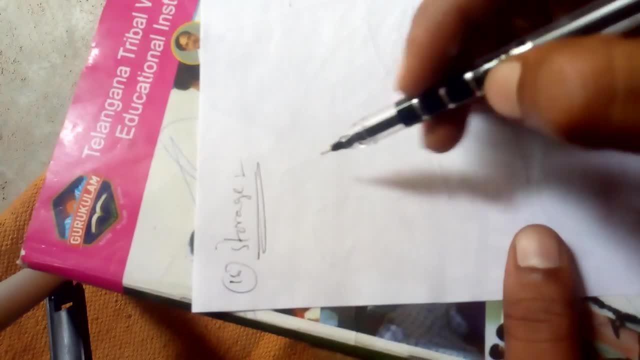 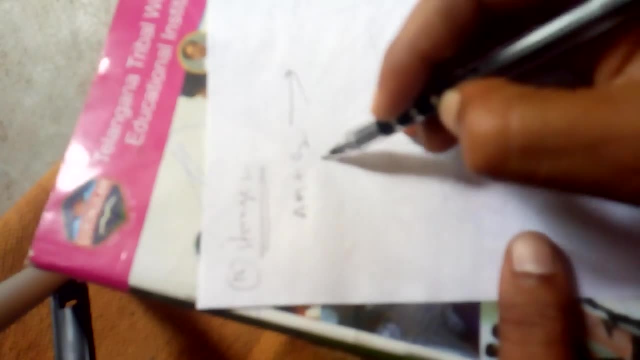 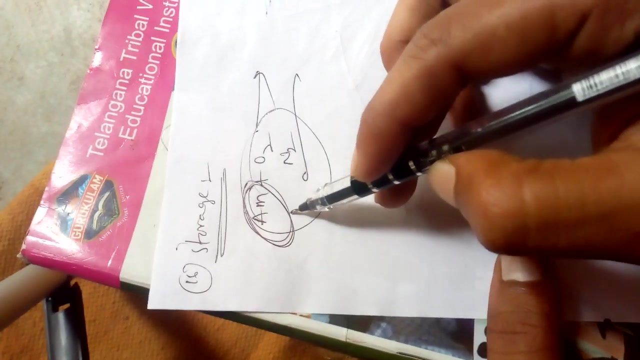 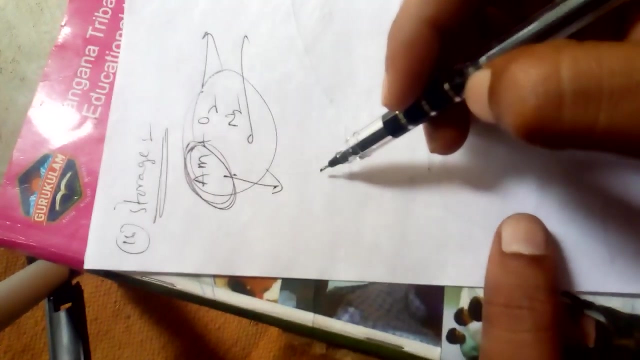 storage when we are discussing about storage, actually, uh, these alkali metals, these alkali metals is reacts with atmospheric air. o2 and endo are everything so atomic. these alkaline, these alkali metals are highly reactive. hence, when they are exposed to atomic uh air, so combined with atmospheric air, it forms 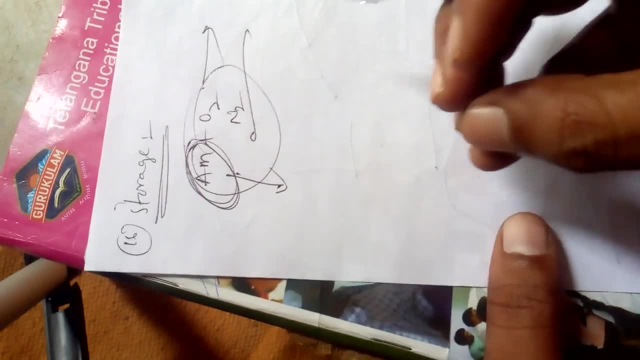 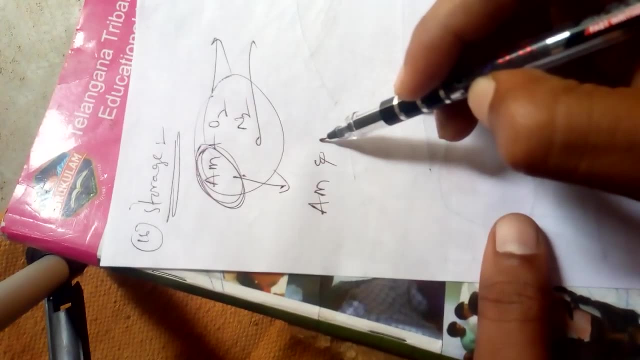 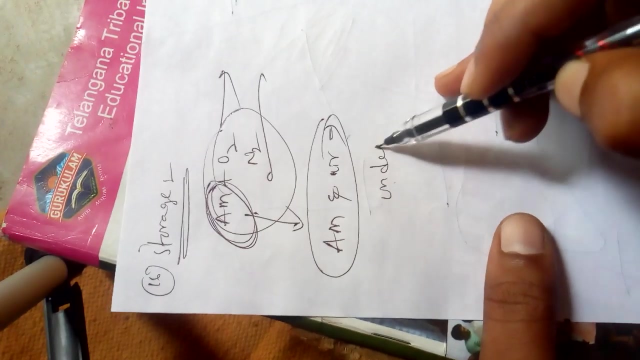 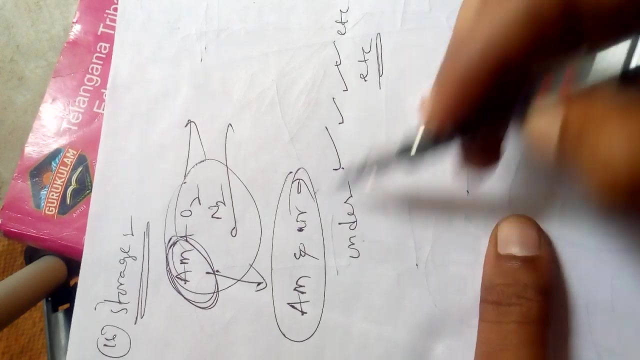 respective compounds, so to to protect or to prevent these reactions between atomic uh, reactions between alkali metals and as well as atmospheric air. so we need to put, we need to store under kerosene or benzene or tolin or petrol, etc. etc. etc. because it reacts with atmospheric air, okay, but 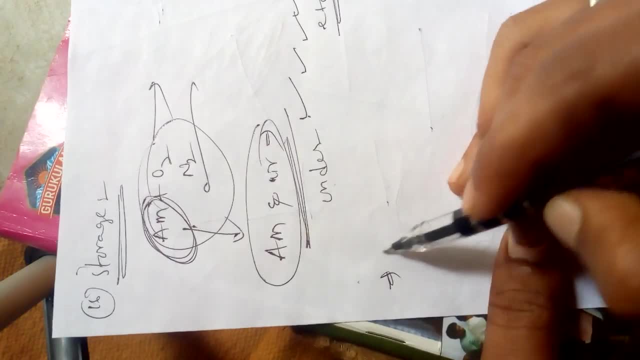 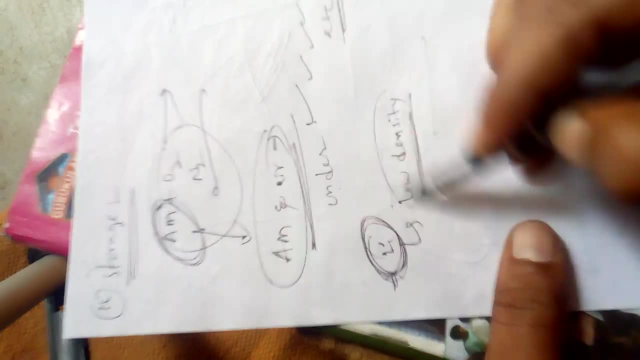 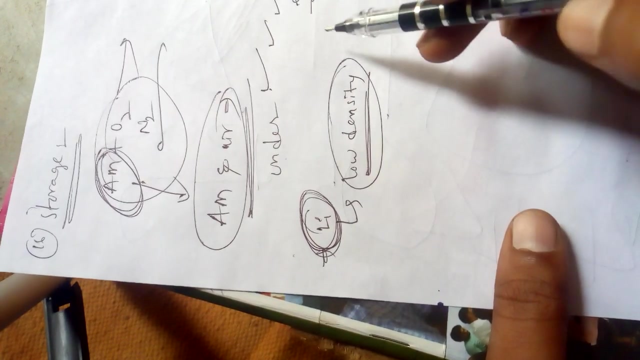 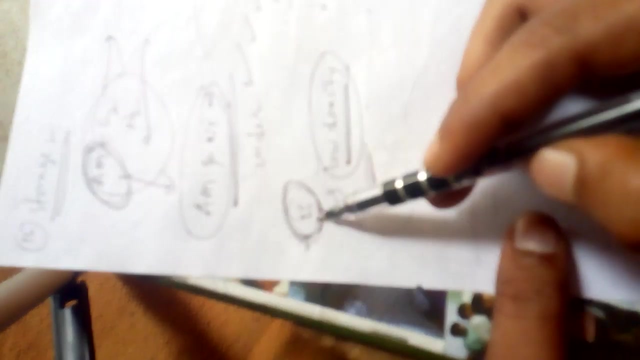 here the confusion and the exception point is like among alkali metals. lithium is having low density. uh, what happens here among alkali metals? except lithium remaining can stored in under these inert solvents, okay, but uh, because of lowest density, the the lithium, the lithium is the lithium.